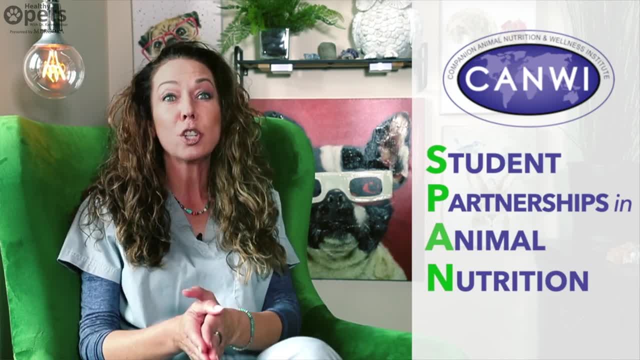 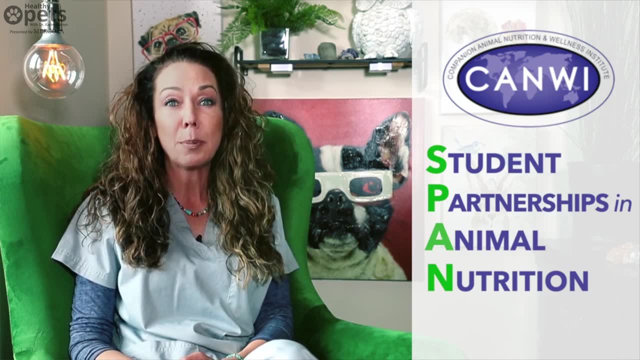 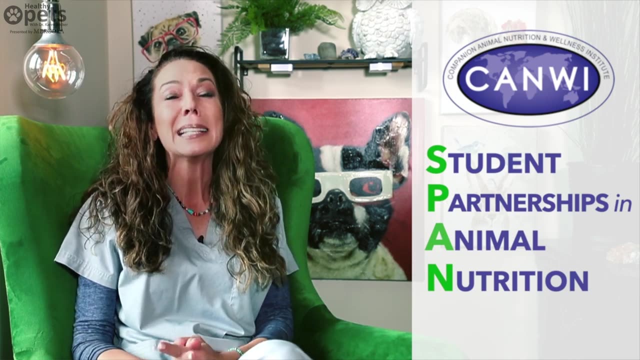 project. It's called the SPAN Partnership or the Student Partnership in Animal Nutrition Program. This innovative program provides veterinary students and vet tech students with educational opportunities to learn about companion animal nutrition from unbiased, board-certified veterinary nutritionists. Enjoy the interview and consider supporting. 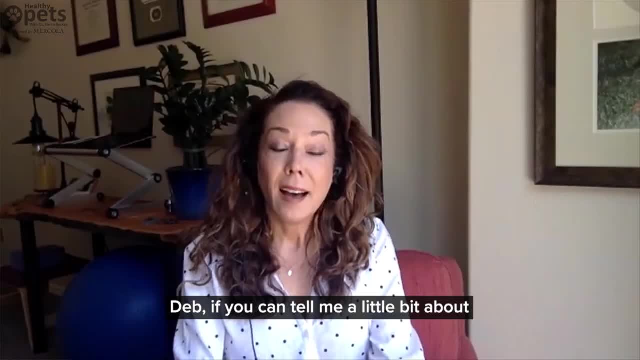 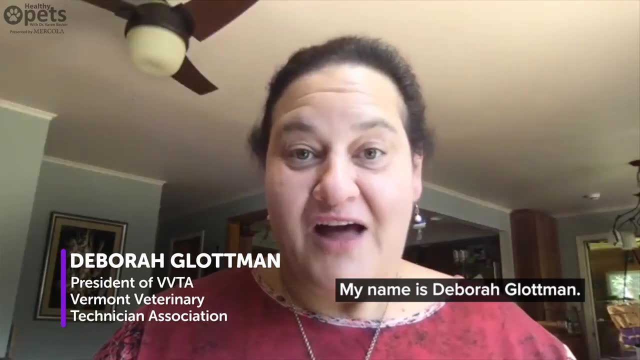 Can We SPAN program this week? Deb, if you can tell me a little bit about who you are and what you do, that would be great. My name is Deborah Glotman and I've been a veterinary technician since 1988.. I'm president of the Vermont Vet. 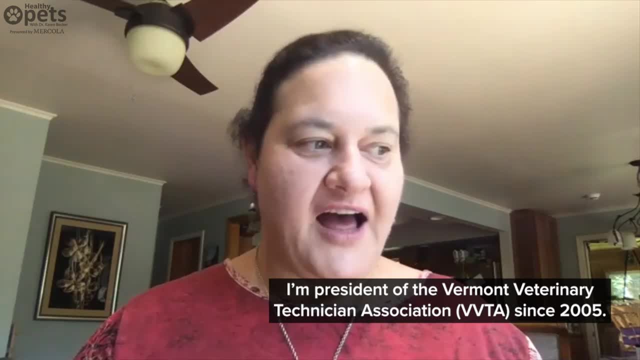 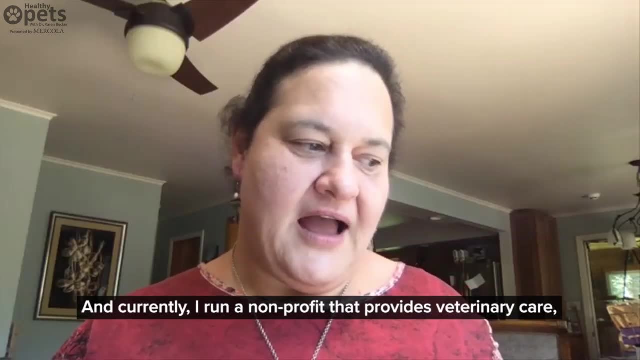 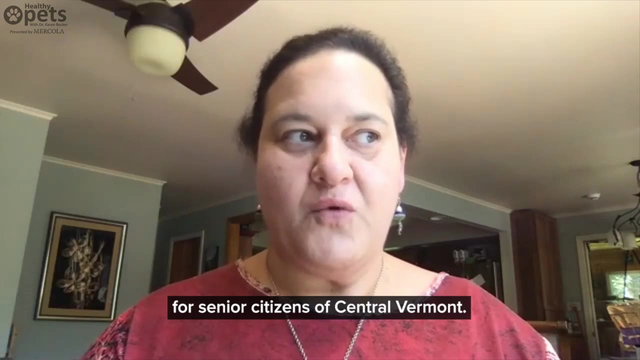 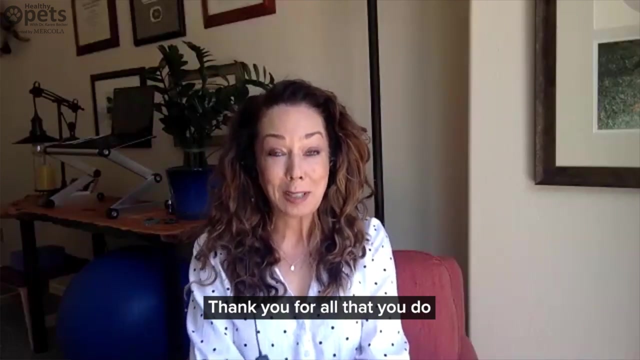 technician association, since I'm an emergency critical care nurse, a surgery nurse, and currently I run a non-profit that provides veterinary care, mostly surgery and dentistry, for senior citizens of central Vermont. Beautiful and wonderful, and thank you for for all that you do in and all of the different realms that you're so passionate about. That's. 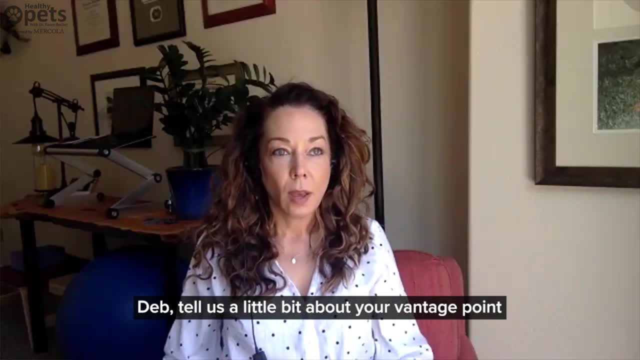 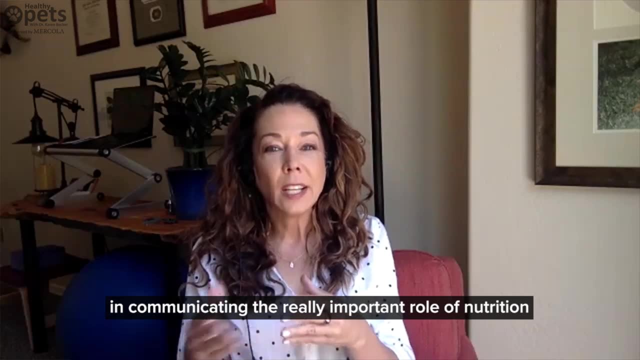 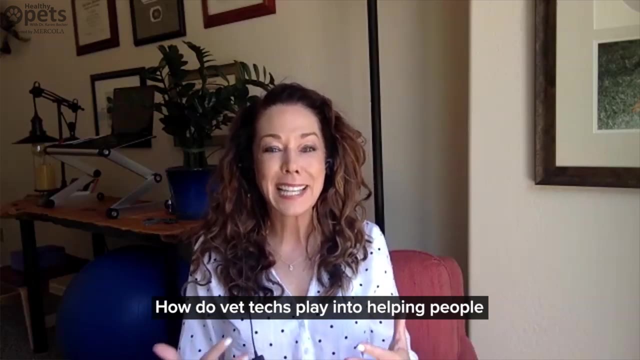 wonderful Deb. tell us a little bit about your vantage point in terms of what roles do certified vet techs play in communicating the really important role of nutrition in an animal's life? in the exam room, How do vet techs play into helping people make better choices? I think 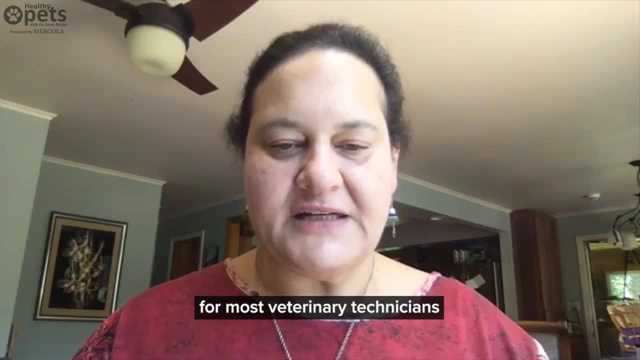 the hardest part for most veterinary technicians is actually getting the time to be able to take that extra minute to discuss the role of nutrition in an animal's life. I think the hardest part for most veterinary technicians is actually getting the time to be able to take that extra minute to discuss. 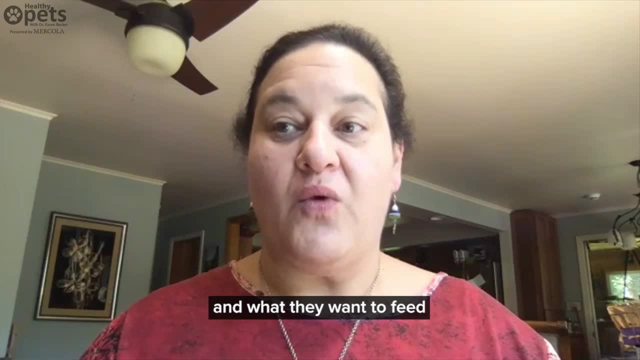 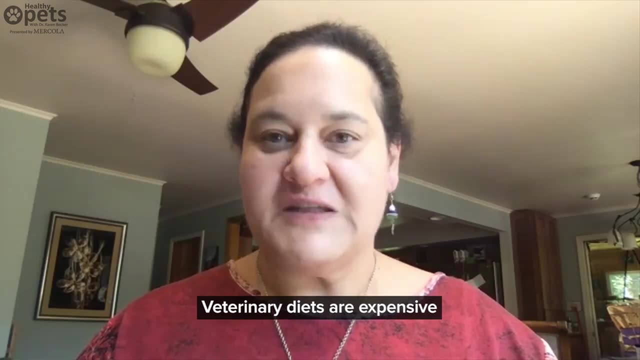 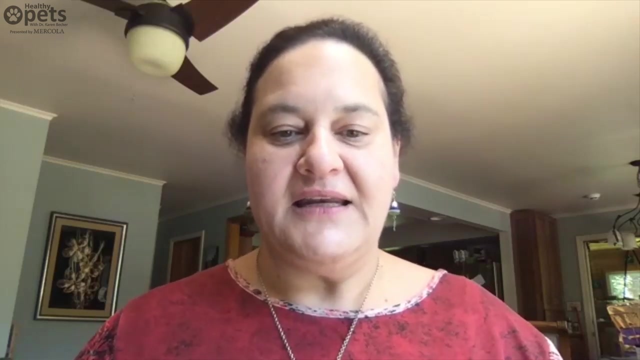 what people are feeding and what they want to feed and what they can't afford to feed. Veterinary diets are expensive and really should be used just for the need of a problem, And then what I wish veterinary technicians would know more to do is proceed to say: well, 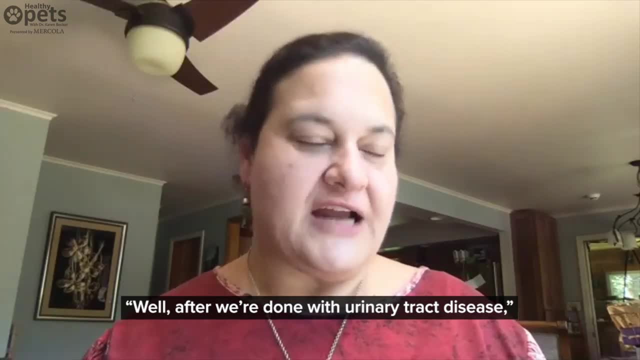 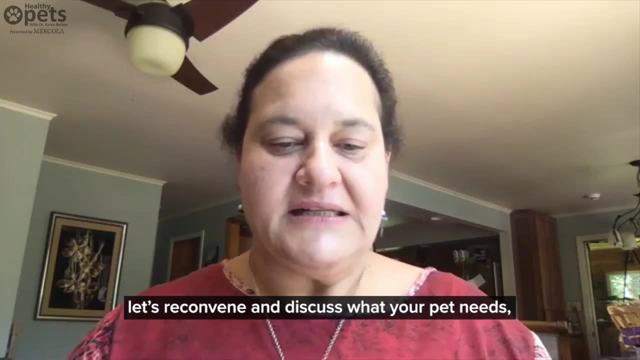 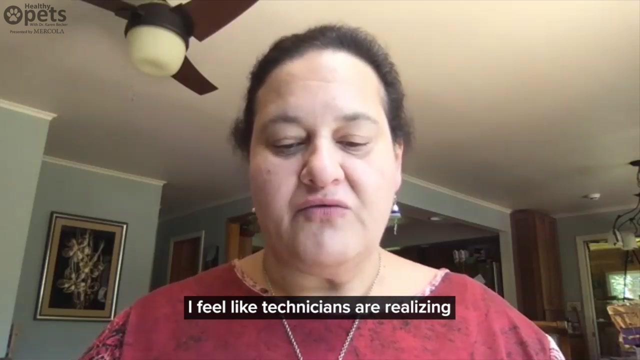 you know, after we're done with urinary tract disease or once we're at a different stage of life, let's reconvene and discuss what your pet needs, depending on what their activity level is, et cetera. So I feel like technicians are realizing and getting better educated, slowly but surely, on 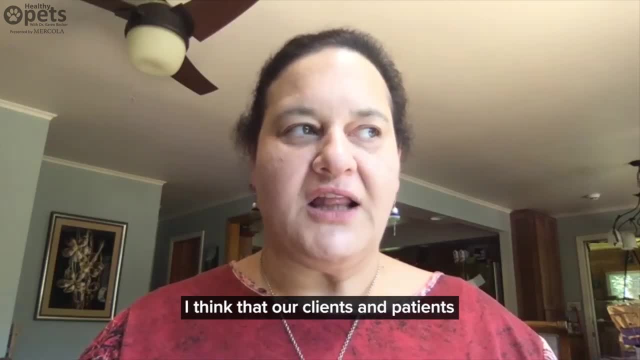 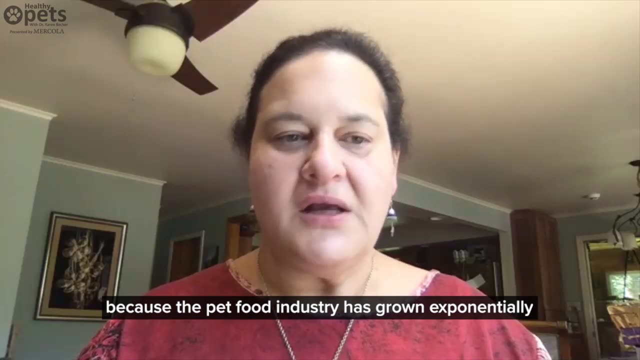 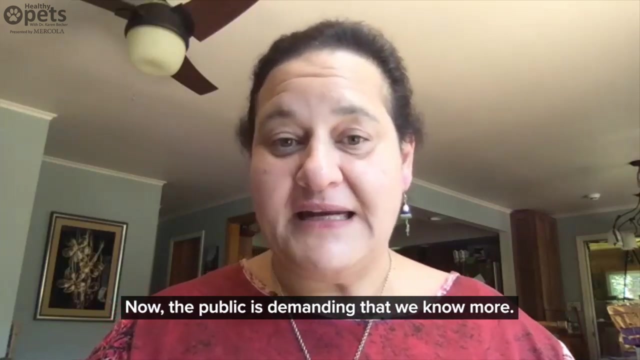 all the needs. I think that our clients and patients are getting such a wide variety of diets because the pet food industry has grown exponentially over the last 10 years. So now the public is demanding that we know more. And you know. think back to when you went. 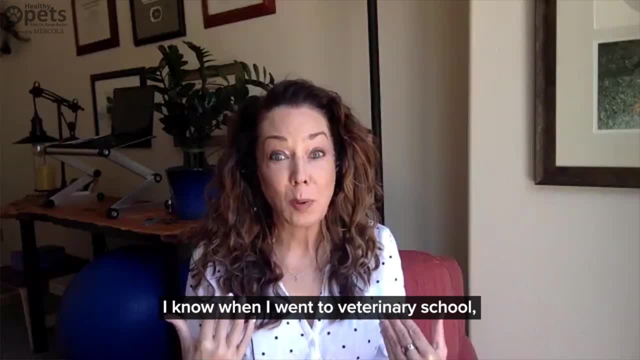 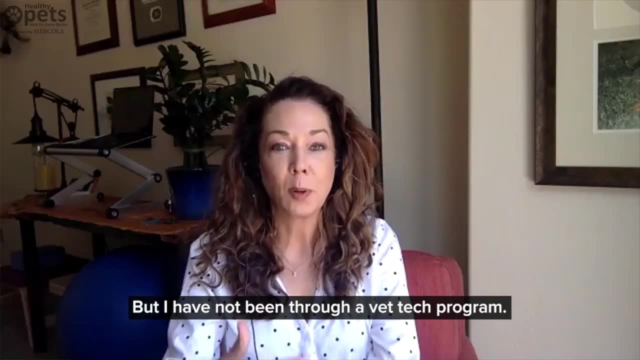 through vet tech training. I know when I went through veterinary school my small animal nutrition education I felt was substantially lacking. but I have not been through a vet tech program. Talk to me about your training. It's you know, usually when I've spoken to. 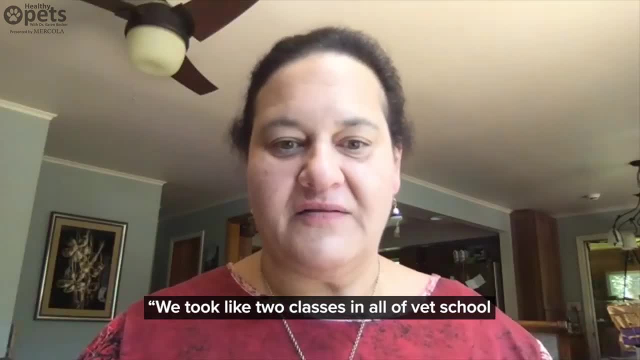 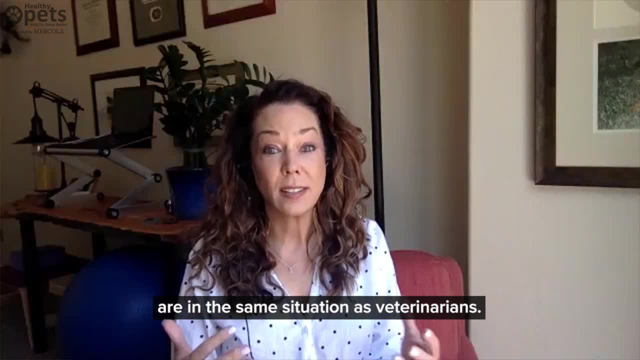 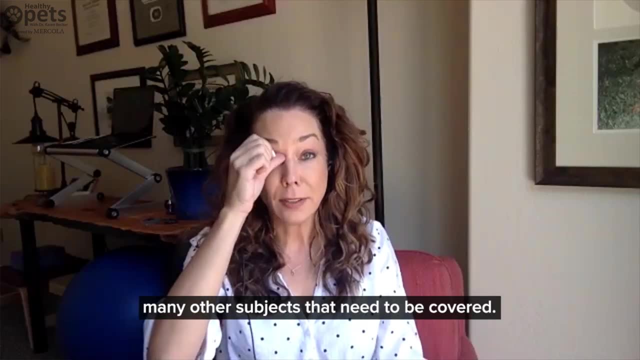 And so it sounds like texts are in the same situations as veterinarians. You know, nutrition really isn't a central focus And, like you said validly, there are many, many other subjects that need to be covered, But I feel, because I'm passionate about nutrition, that nutrition is. 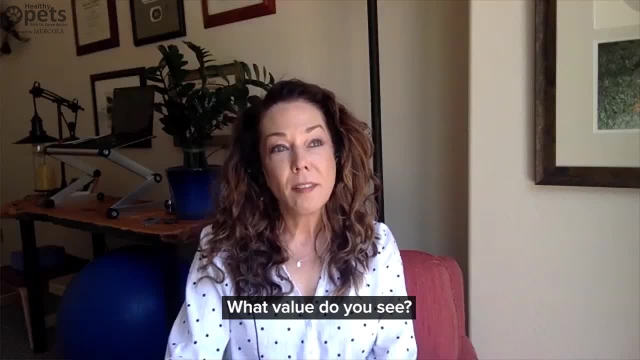 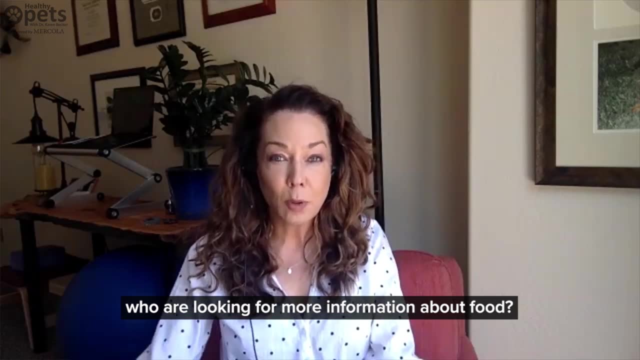 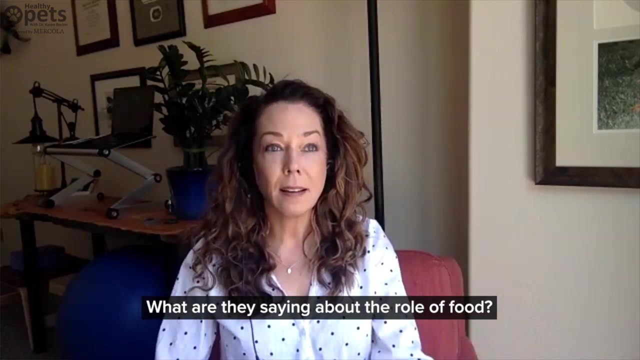 oftentimes left behind. What value do you see or what are students saying? Do you have some students that are looking for more information about food? We have a younger generation than when we went through. What are they saying about the role of food, or are they interested in learning more about? 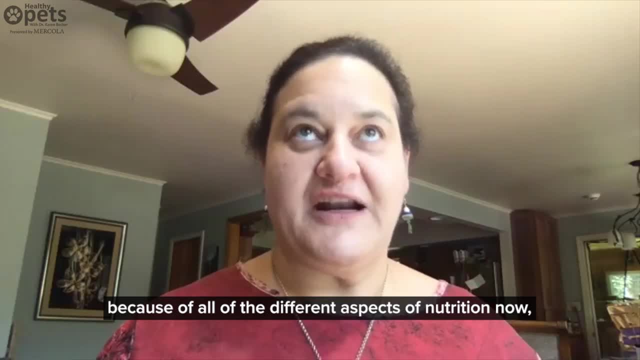 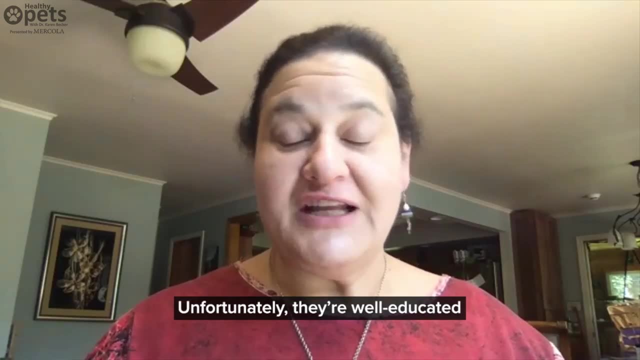 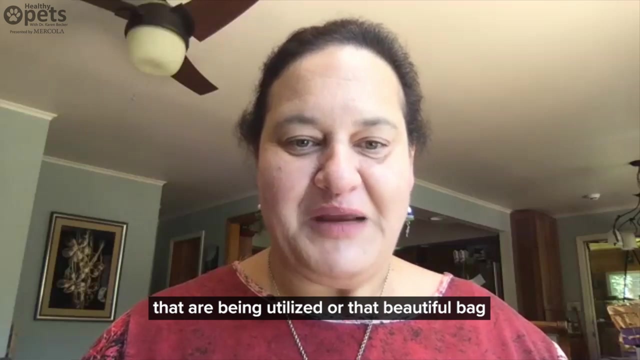 food. I definitely because of all of the different aspects of nutrition now that clients are so well educated in- and unfortunately they're well educated by the pet store employee- or the awesome commercials that are being utilized, or that beautiful bag that you know points. 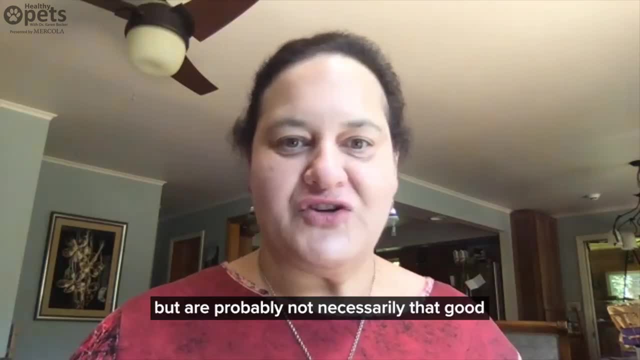 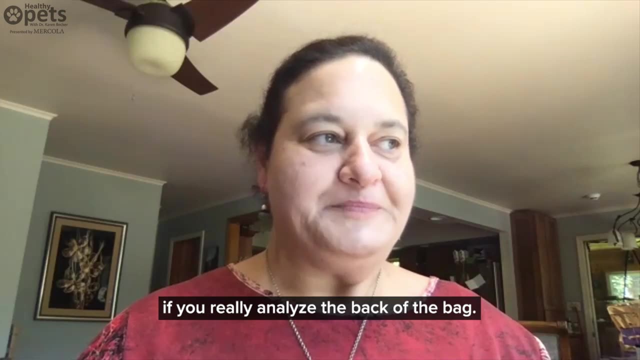 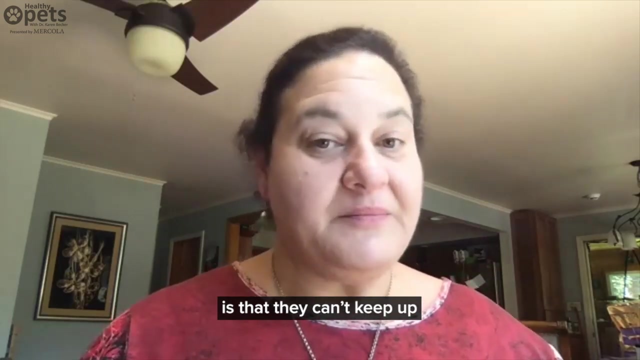 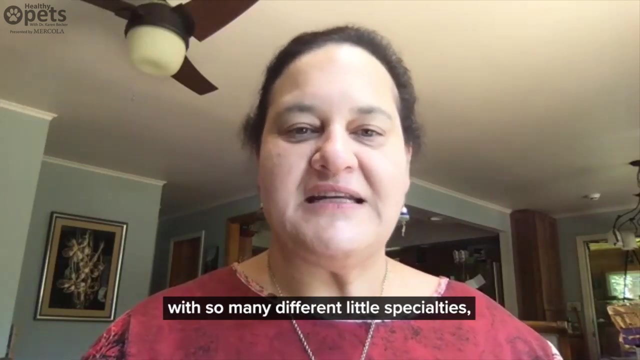 out all of the good things by pictures, but are probably not necessarily that good if you really analyze the back of the bag. So what I'm hearing from technicians and from students is that they can't keep up because the pet food industry is selling so much with so many different little specialties. whether 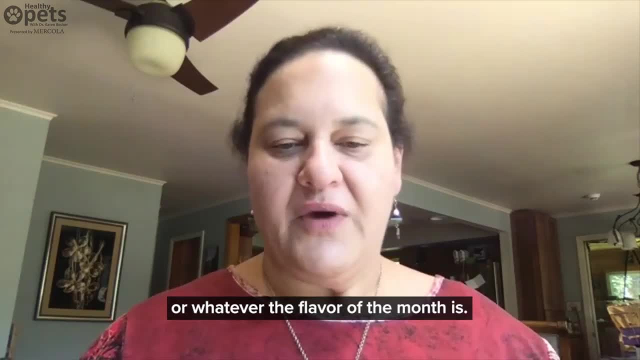 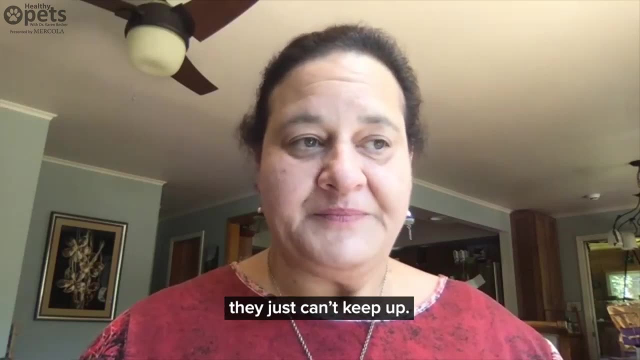 it be raw or Or grain-free or you know, whatever the flavor of the month is that technicians and veterinarians, they just they can't keep up. So it's really important that everybody look at the entire picture and not just the little. 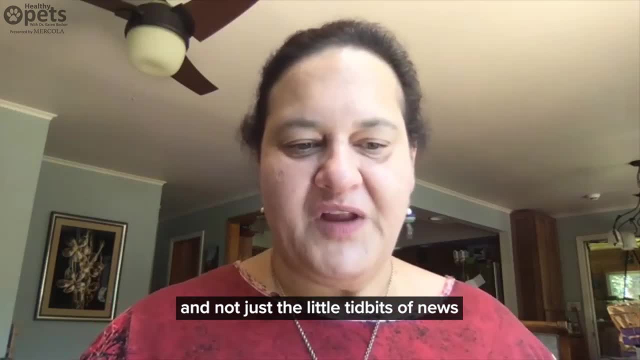 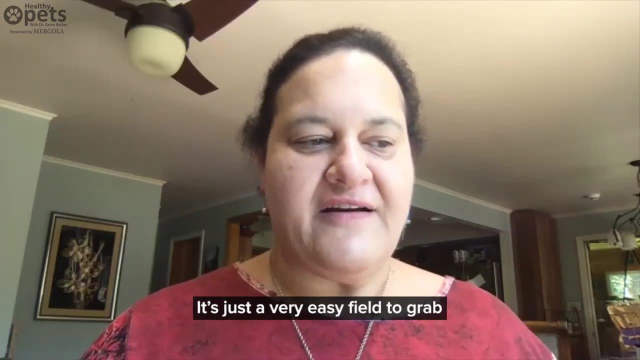 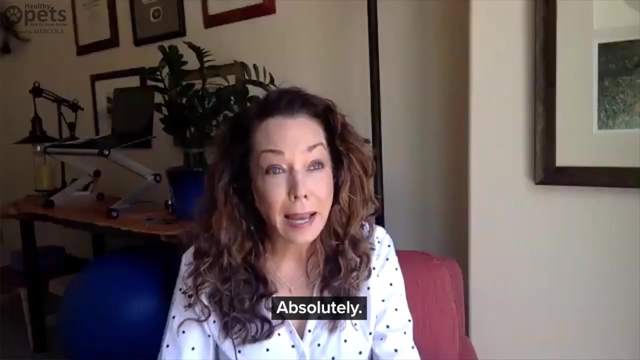 you know tidbits of news that they're getting on Facebook, or you know it's just, it's a very, it's a very easy field to grab a little bit of knowledge and make a whole lot of damage. Yeah, absolutely. 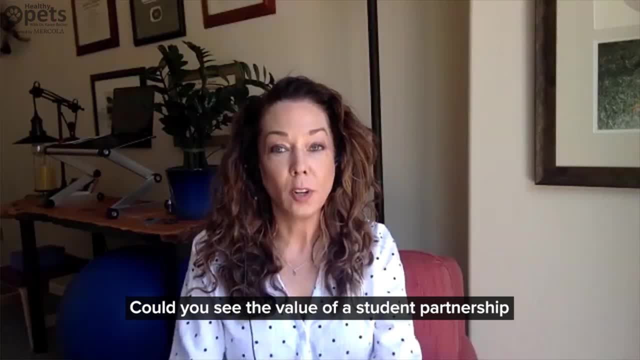 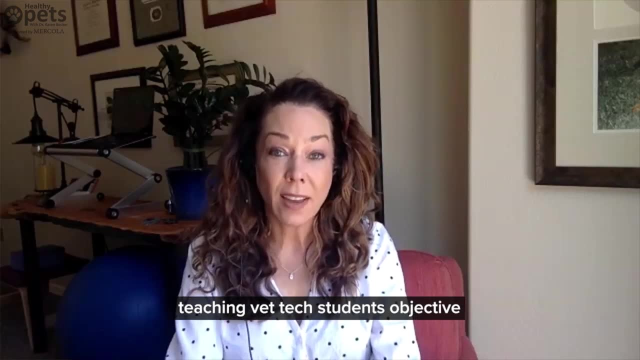 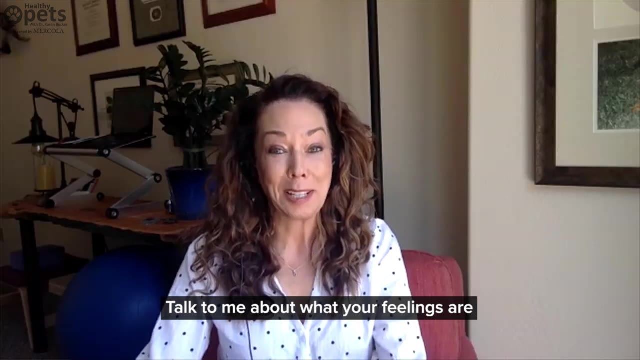 And so could you see the value of a student partnership in animal nutrition, the value of having a board-certified nutritionist teaching vet tech students objective: small animal nutrition. Talk to me about what your feelings are if that were to be instituted in vet tech programs. 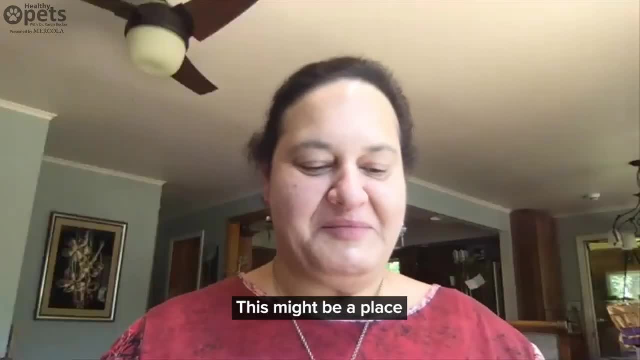 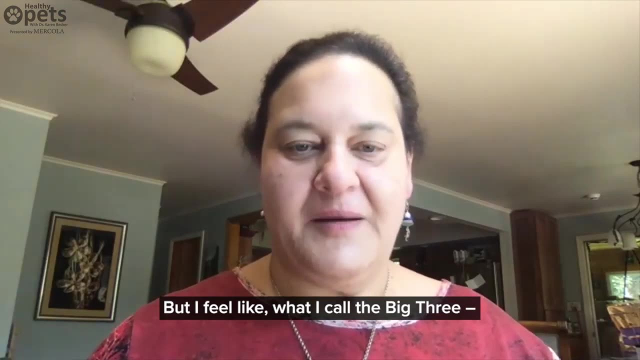 nationwide. So this might be a place that not everybody feels the same way as I do, But I feel like the what I call the big three Hills- Purina and Royal Canin. I feel like they get a lot of time in front of most of these students and veterinary students. 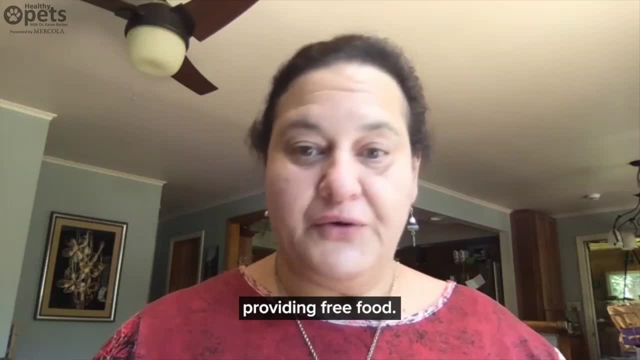 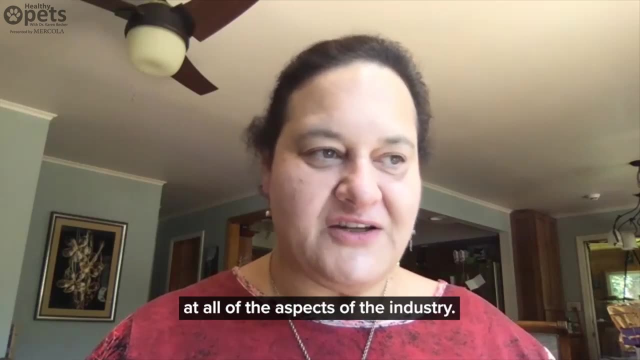 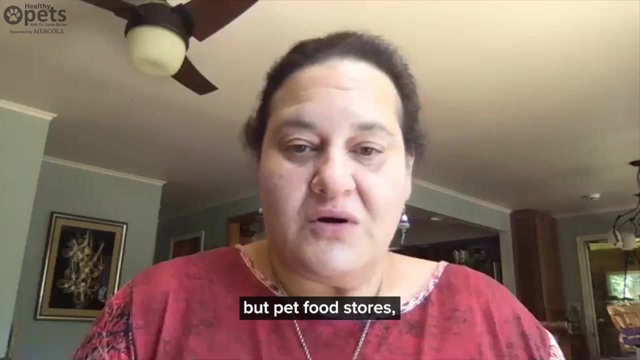 because they're also providing free food And I and I get that and I know that they appreciate it. but I do feel like we have to look at all of the aspects of the industry. You know, we, if you walk into some not just boutique but pet food stores, like 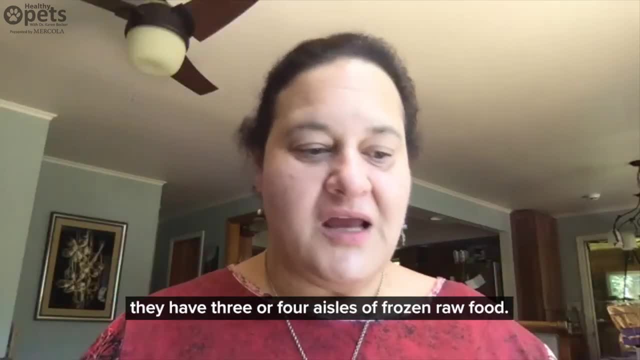 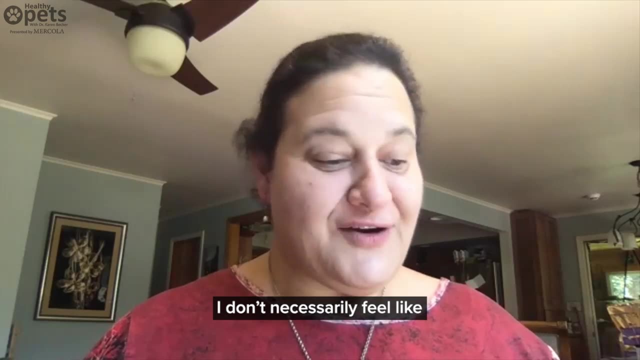 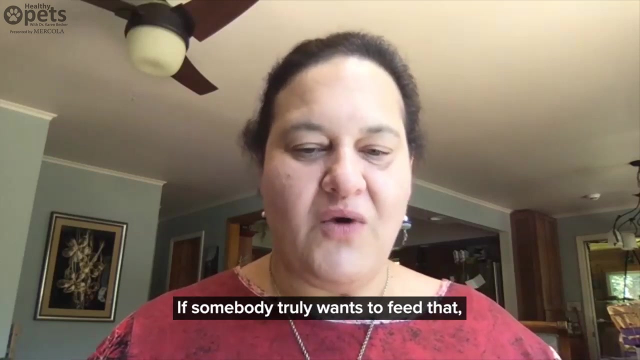 you know all the national big box stores. you know they have three or four aisles of frozen raw food. I don't necessarily feel like raw is an answer to anything, but I feel like we need to be educated in it And if somebody truly wants to feed that, then we should at least know every aspect. 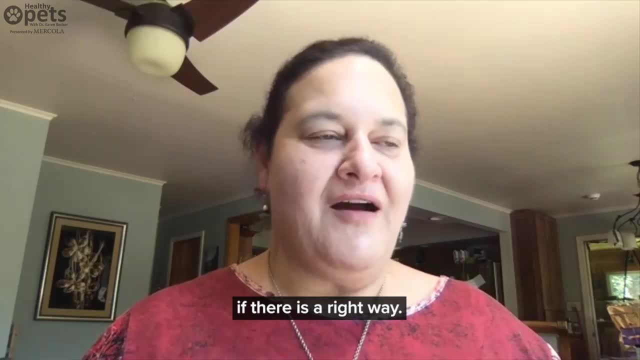 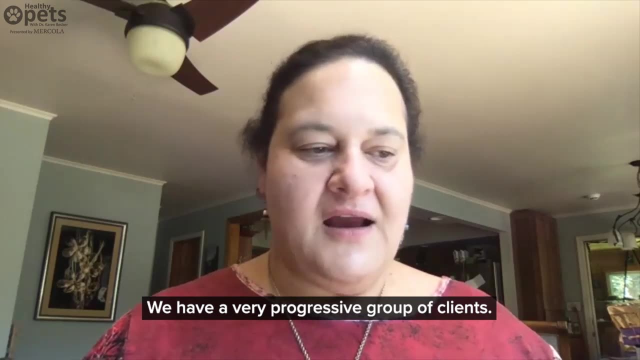 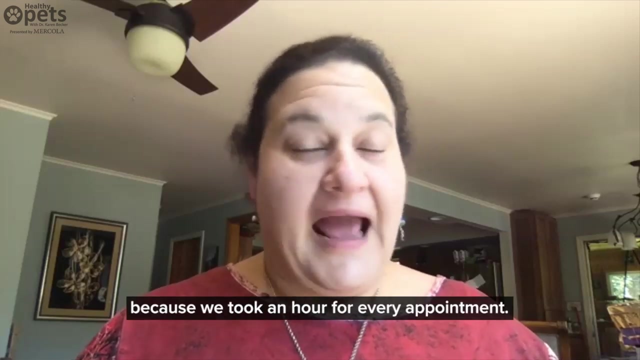 of the right way of doing it, If there is a right way. I live in Vermont and we have a very progressive group, And so you know we have a lot of clients. my practice was what we almost called a concierge practice, because we took an hour for every appointment. 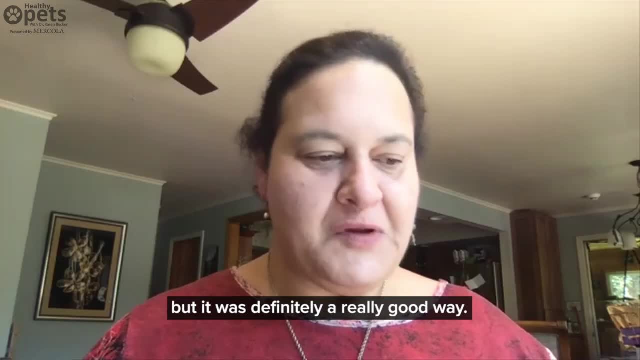 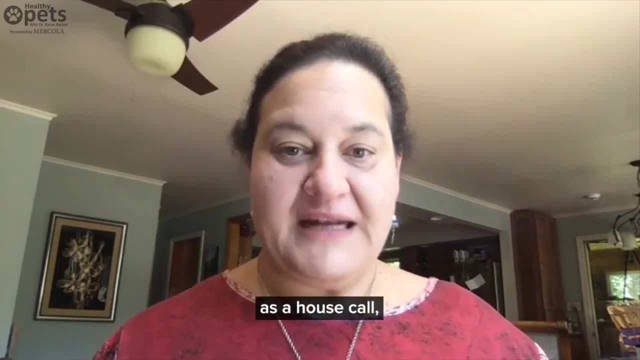 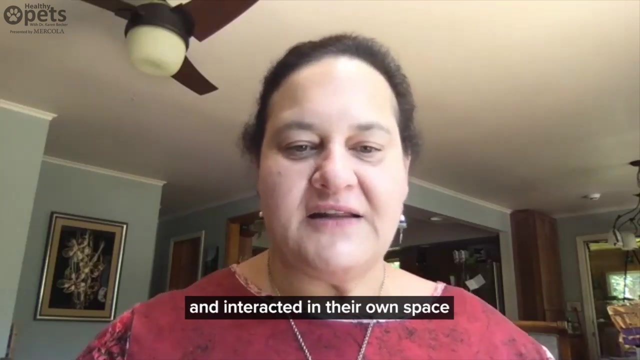 And that is, by the way, not fiscally responsible, but it was definitely a really good way. Often we would do our first appointment as a house call, so we could see how all of the animals lived and where they lived and how they lived and interacted in their own space. 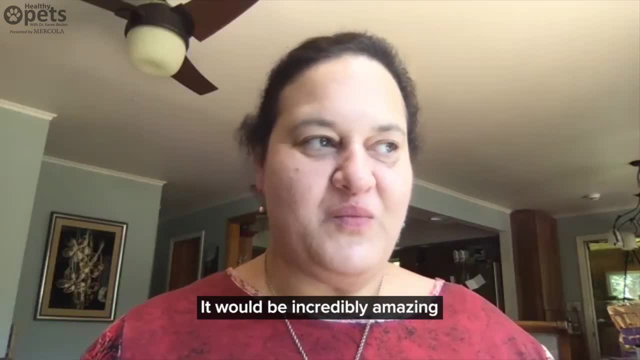 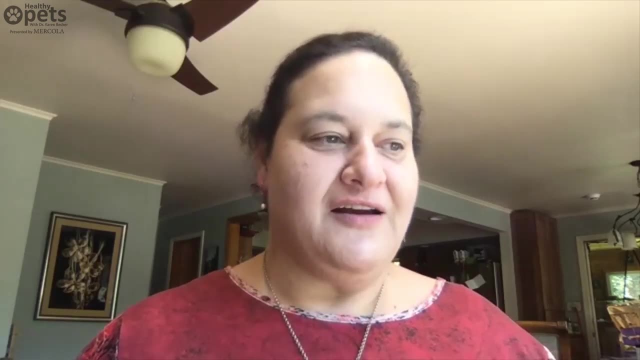 And what they were getting to eat. you know it would be incredibly amazing to watch how many times a client gives a treat. you know come sit, come in, go out. you know all these different aspects that they don't realize. calories are coming in and not going out in. 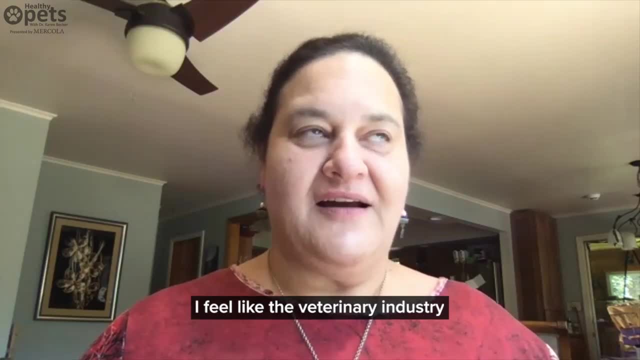 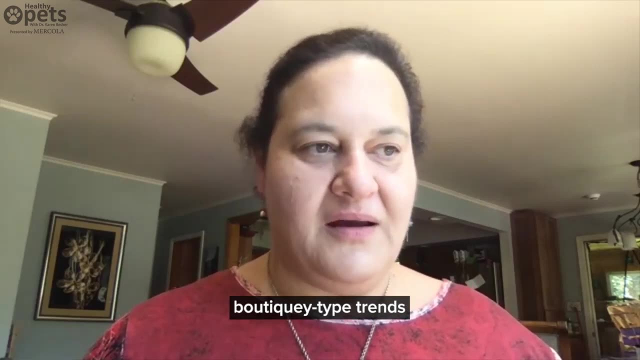 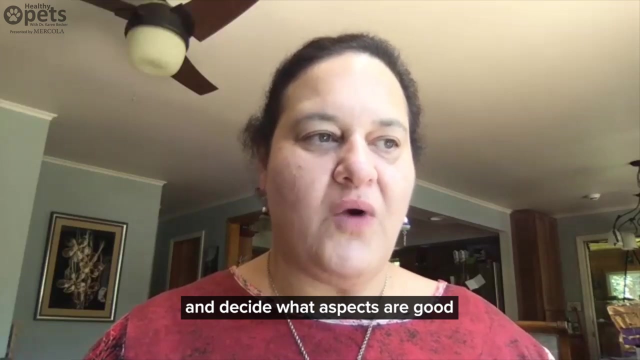 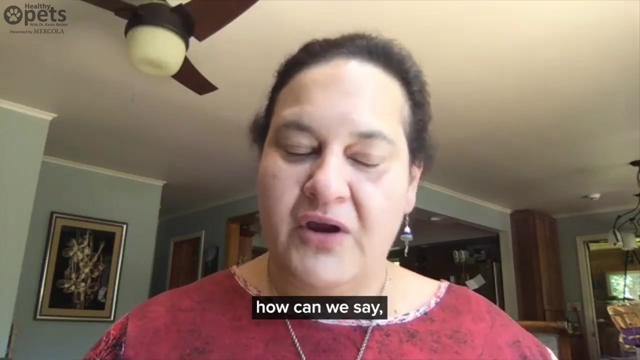 any other way. So I feel like the veterinary industry needs to realize that all of these boutique-y type trends are here to stay And if we don't get well-versed in them and decide what aspects are good and what aspects are bad, and if somebody insists on feeding it, how can we say: all right, if you insist. 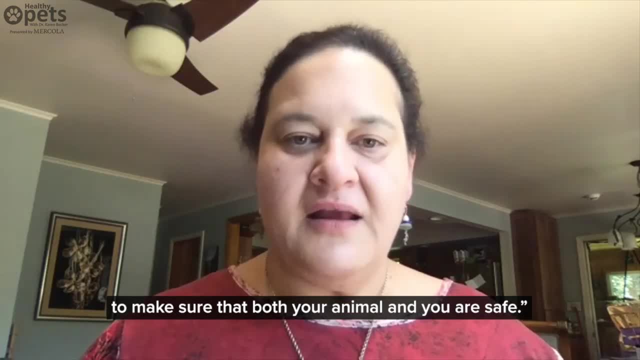 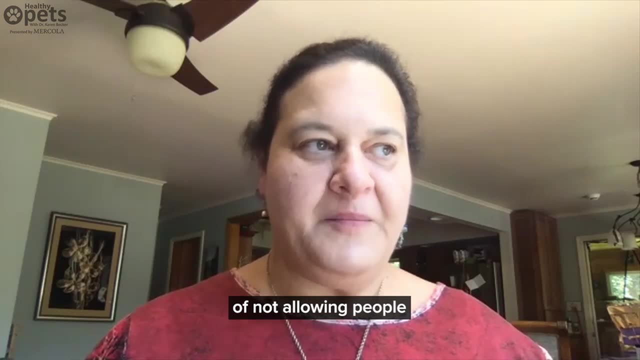 on feeding this. at least do this, or at least do that, to make sure that both your animal and you are safe. I feel like we're always fighting the fight of not allowing people or trying to talk them out of things When we have them fight. 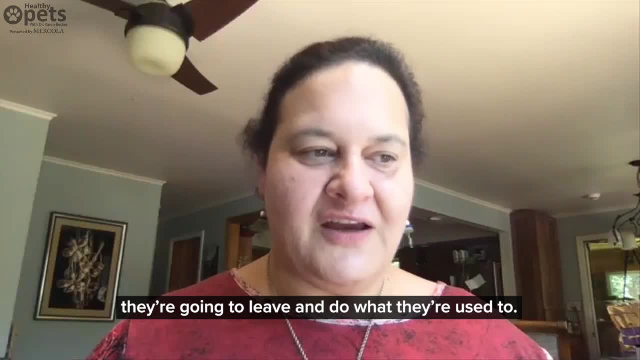 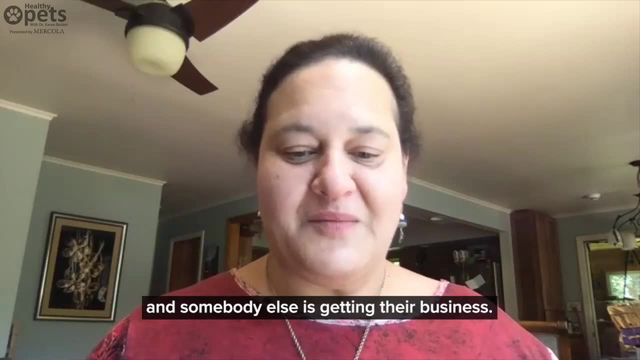 For 15, 20 minutes in an exam room. they're going to leave and do what they're used to, So at least give them good advice on what we know they're going to do, because somebody else did and somebody else is getting their business. 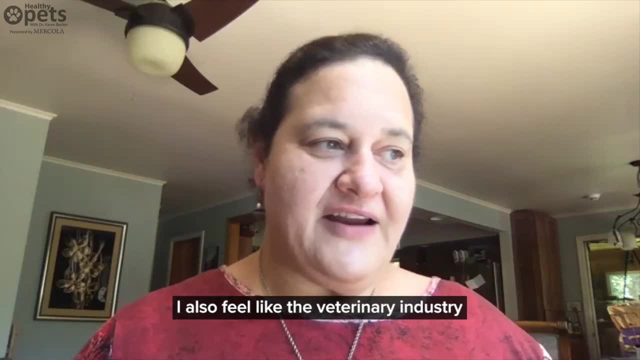 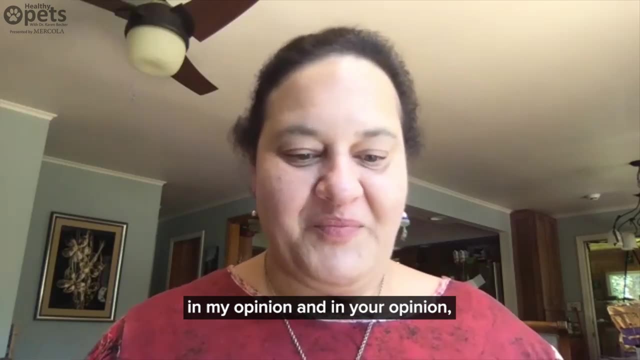 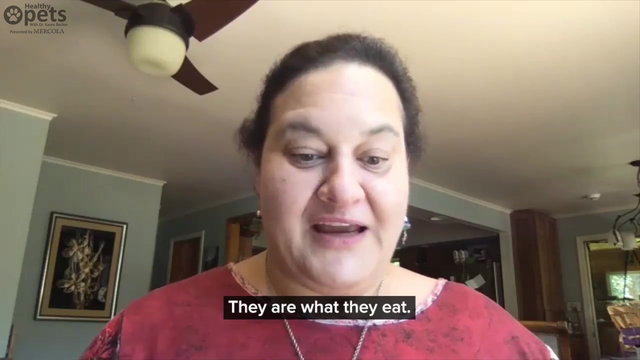 And I also feel like the veterinary industry needs to decide that nutrition is, in my opinion, in your opinion. you know, it's the core of absolutely everything That animals. they are what they eat, Their blood work is what they eat. 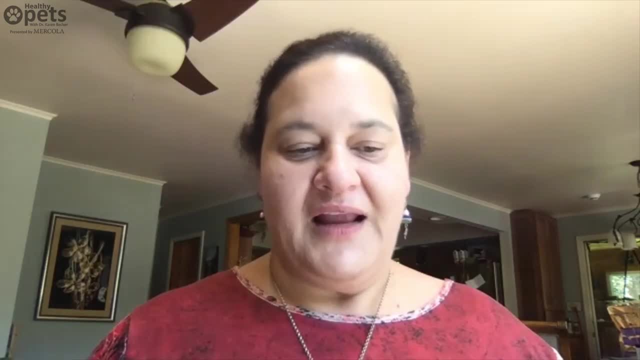 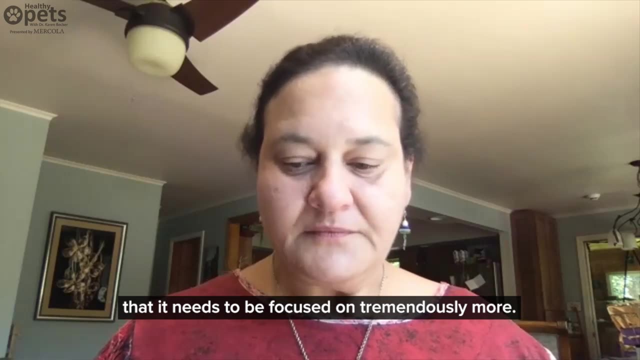 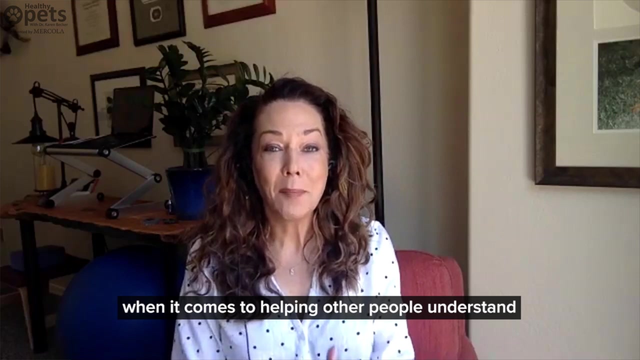 Their medical issues are what they eat, And I think, just like yourself, that it needs to be focused on tremendously more Well. I appreciate your valuable insights. I appreciate you offering your wisdom when it comes to helping other people understand where we're at as technicians and veterinarians, trying desperately to help people understand. 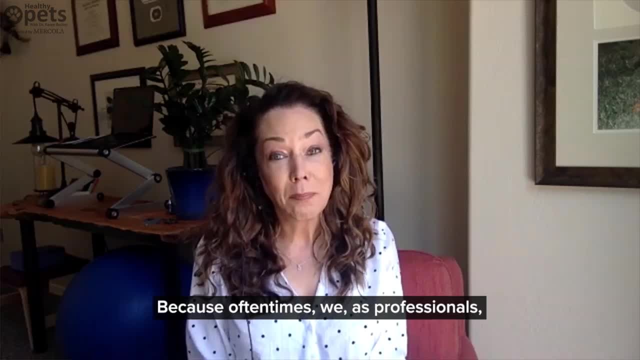 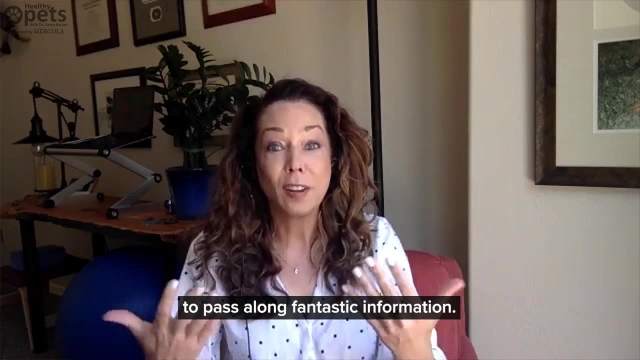 and help our clients understand the value of nutrition. But it's hard because oftentimes we as professionals aren't necessarily trained in a way that provides us all of the background we need to pass along fantastic information. Hence us wanting to get the word out. 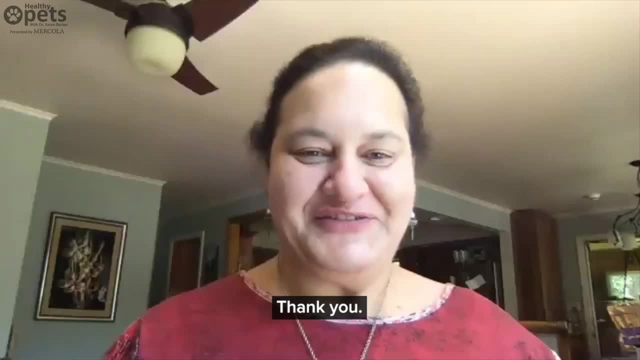 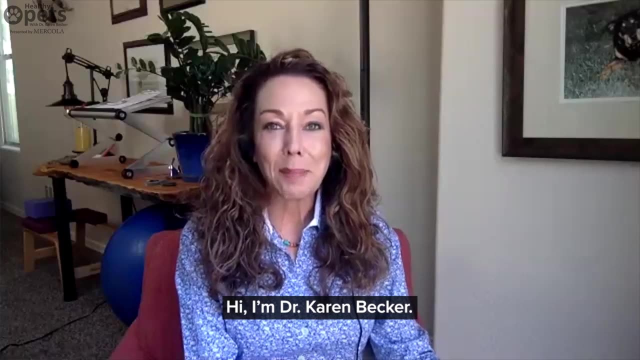 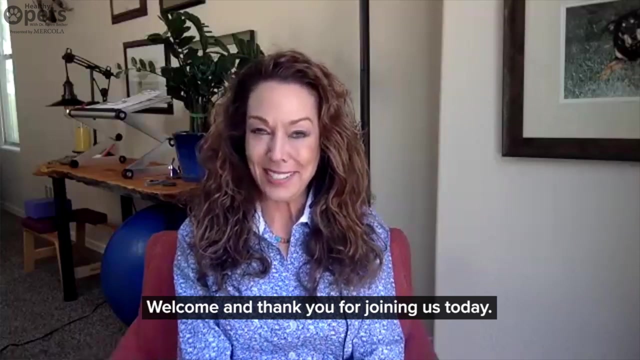 We appreciate everything you're doing, Deb. Thanks so much. Thank you, Hi. I'm Dr Karen Becker and I'm interviewing veterinary technician educator Heather Darma McClellan. Hello, Hello, Heather, and welcome for joining us today. 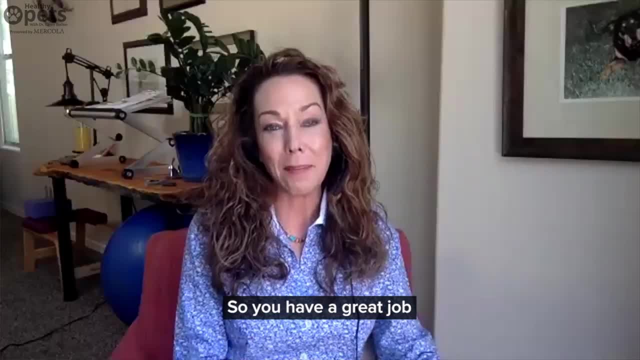 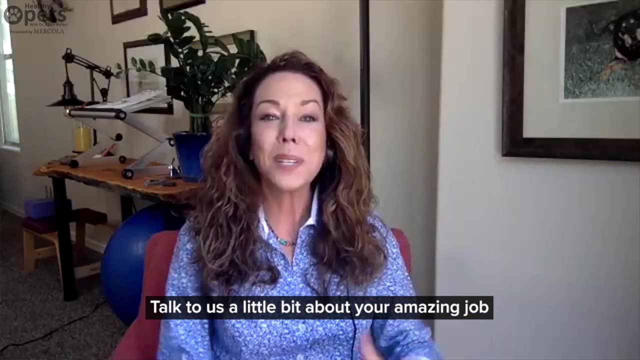 Thank you, Dr Becker. This is really great. So you have a great job in that you are a certified vet tech, but you are in academia doing teaching, educating, right now. So talk to us a little bit about your amazing job that you have, and then also how you're. 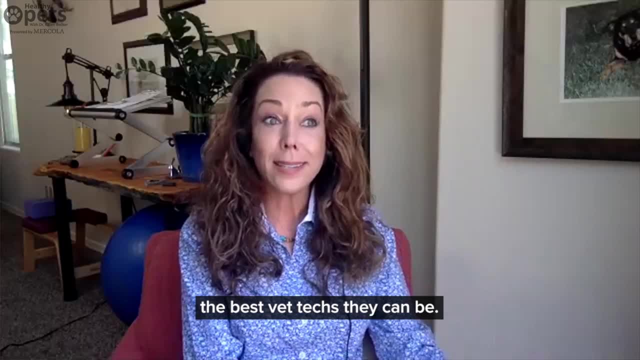 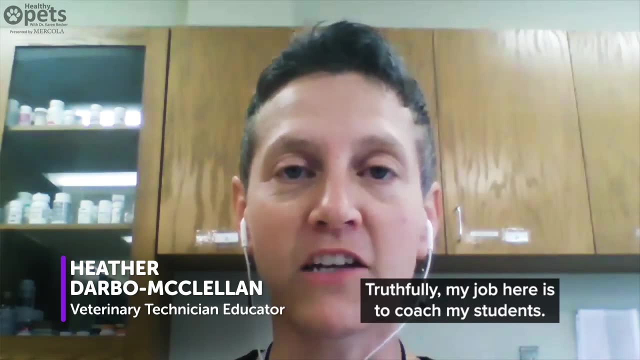 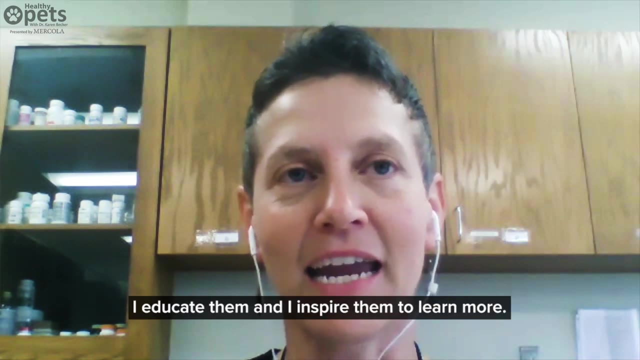 really committed to helping other students learn to become the best vet techs they can be Absolutely Well. I love educating, training and inspiring And, truthfully, my job here is to Coach my students. I give them the information, I educate them and I inspire them to learn more. 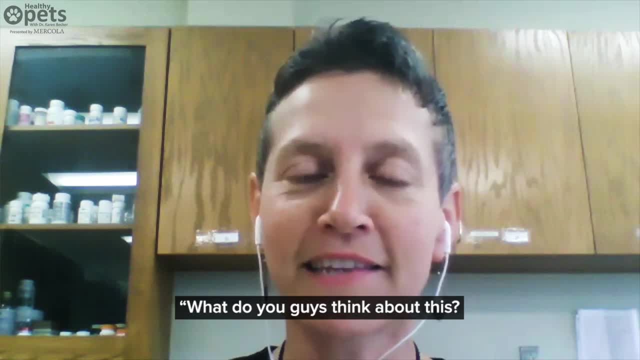 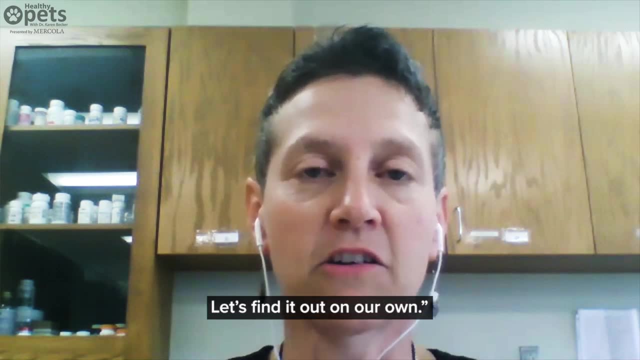 So a lot of my teaching and conversations are: what do you guys think about this? What have you heard out there in your own pets, What have you heard out in the industry And what would you like to know? And let's find it out on our own. 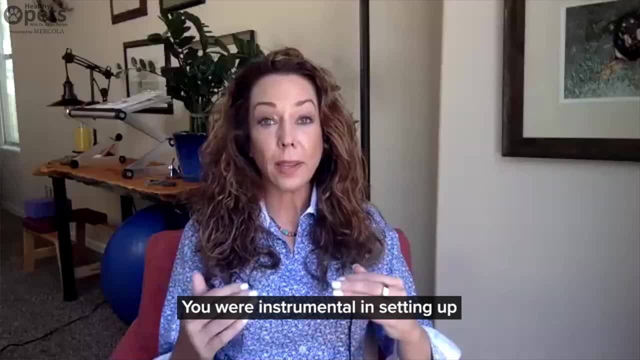 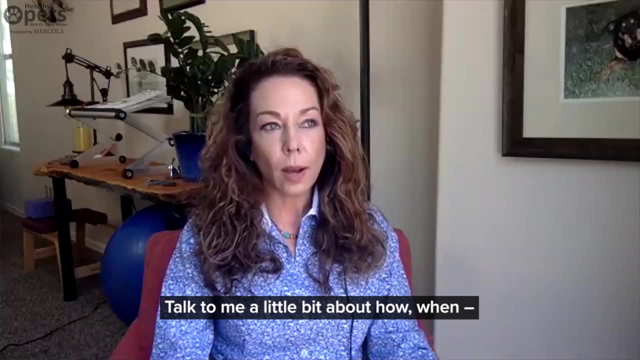 Yeah, And so talk to me a little bit about you- were instrumental in setting up this brand new vet tech program, So talk to me a little bit about how. So it's called Gateway, and so talk a little bit about what Gateway is. and then how do? 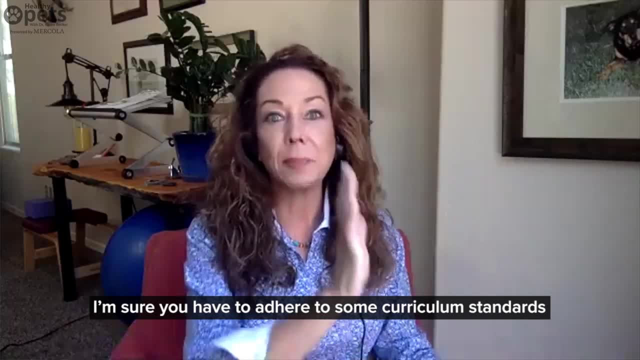 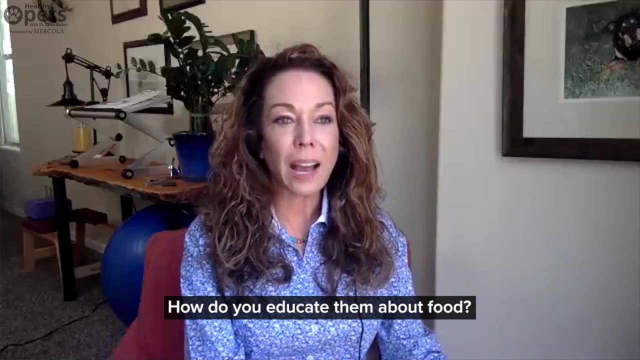 you choose your, I'm sure that you have to adhere to some curriculum standards for how you pick it. but how do you decide how to educate the veterinary technician students that come into your program? How do you educate them about food? Well, our program is again. it's accredited. 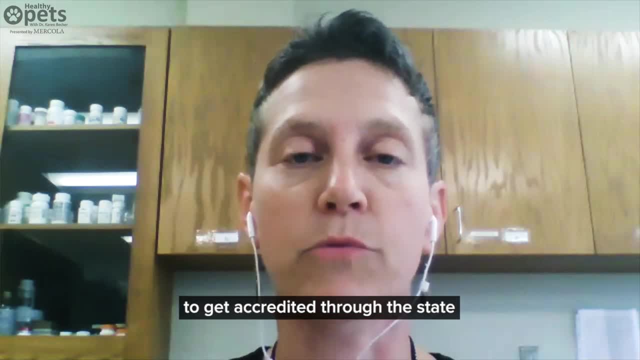 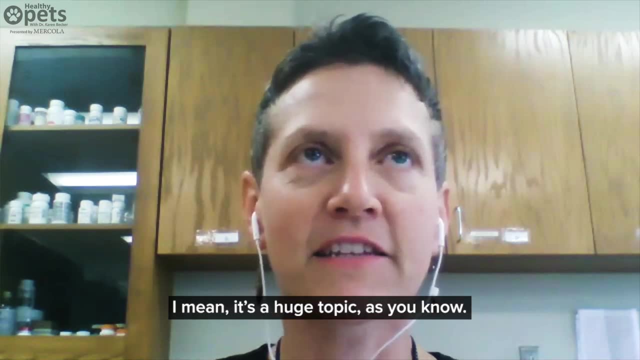 So we have gone through all the processes to get accredited through the state for a vet tech program And the information that we have for nutrition is, I mean, it's a huge topic, as you know, And we literally are encouraging the students to say: you know, here you have a pet. 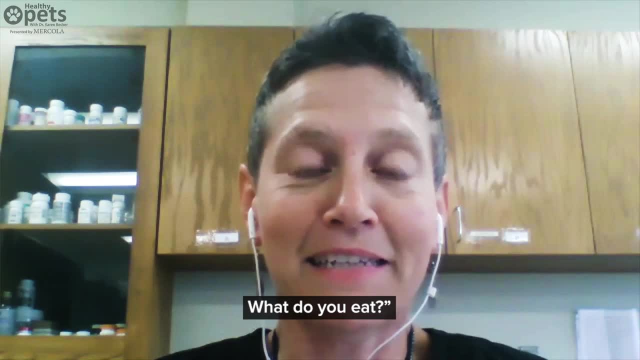 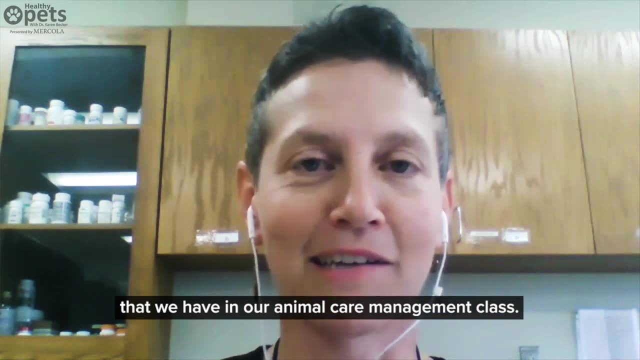 What do you feed your pets, What do you eat? And our conversation is almost one of the biggest debates that we have in our animal care management class. Yeah, I believe that. And Heather, are you finding over the? You've been a tech for a long time. 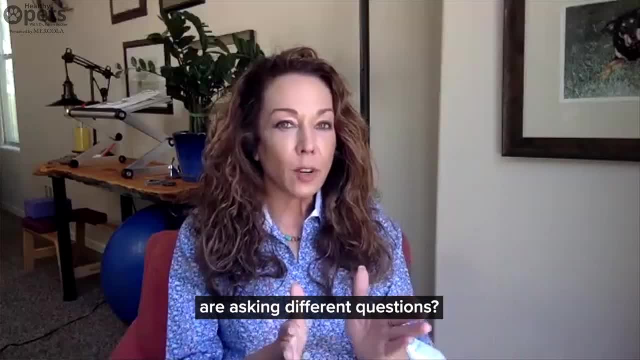 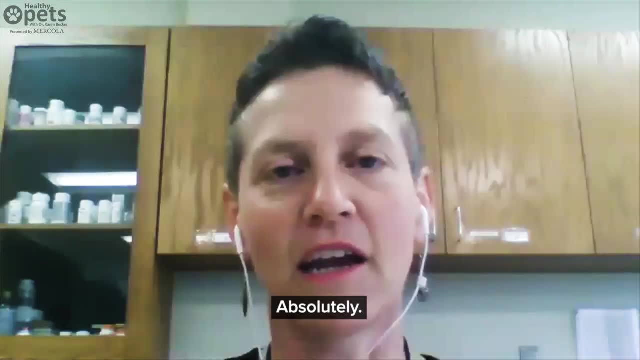 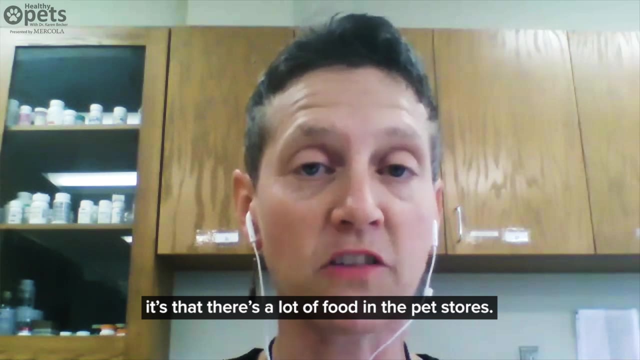 Are you finding that your students? Are you finding that your students? Are you finding that your students, Your students, are asking different questions? but also, in practice, are you finding that pet parents are asking more questions about nutrition? Absolutely. I mean again, like we've seen, is that there's a lot of food in the pet stores and there's 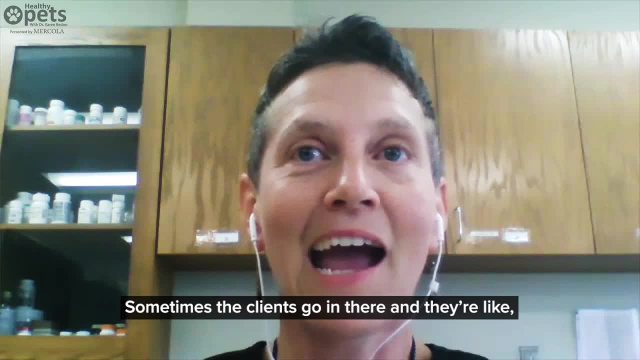 a lot of options And sometimes the clients go in there and they're like I don't even know what to pick. There's too many options. What do I find out? And a lot of the stuff that they find out is on the internet. 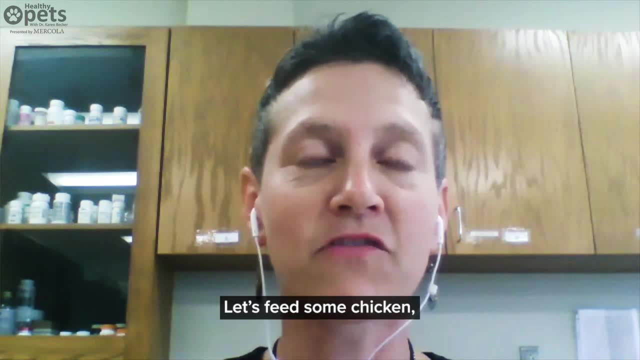 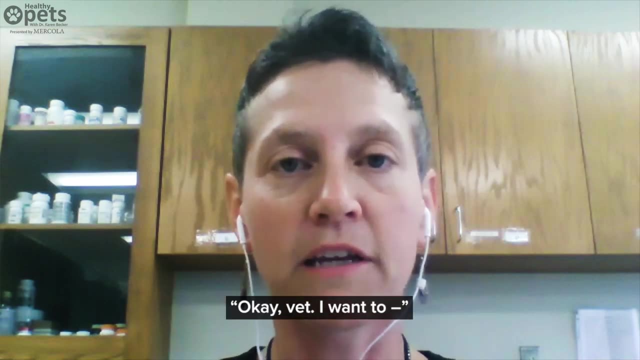 So they may be saying, okay, I want to feed raw, Let's feed some chicken, just raw chicken, And that's not adequate. But then they go to their vet and they say, okay, vet, I want to. Their veterinarian may not have as much knowledge about raw diet. 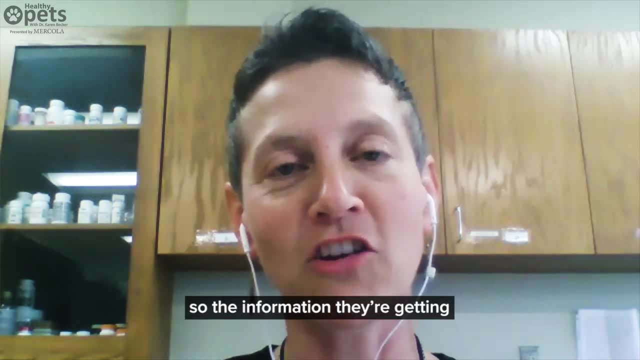 So he's like: well, don't feed raw, But they still want to, So the information they're getting is not from the best resources. So as my students come in, I'm like, okay, let's start looking into this. 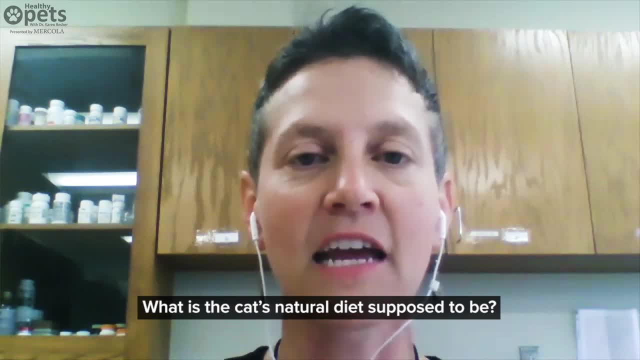 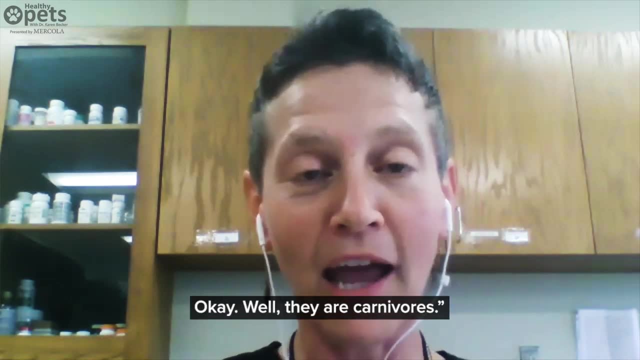 What about behaviorally? What is a cat's natural diet supposed to be? Let's look at lions. Let's look at tigers. What do they eat? Okay, Well, they are carnivores. And then the next thing we do is what? 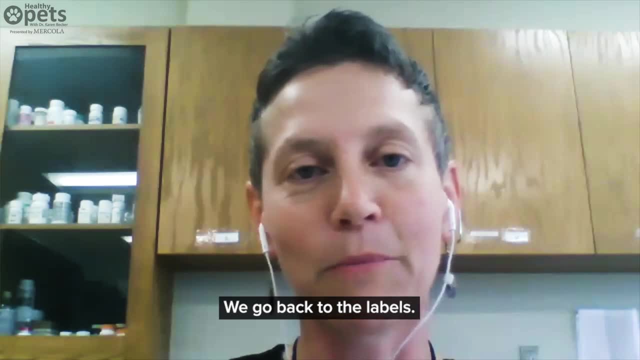 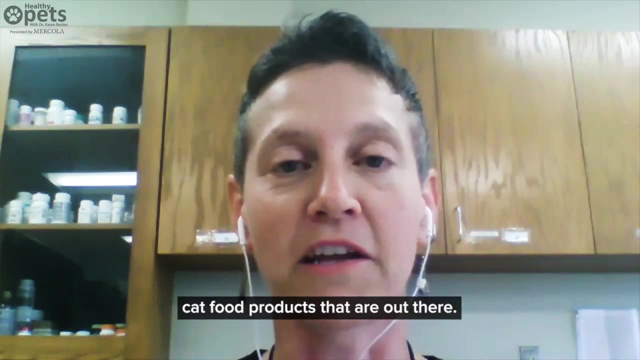 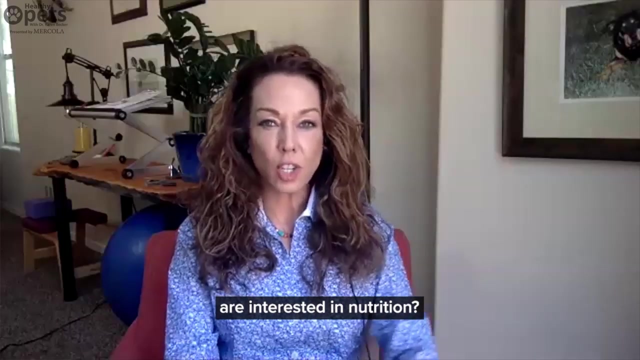 Look at labels. Yeah, I mean, we go back to the labels and you see right there that carnivorous nutrition is not most of the dry cat food products that are out there. And do you find that your students are interested in nutrition, Or does it? I mean, does it feel to you like? 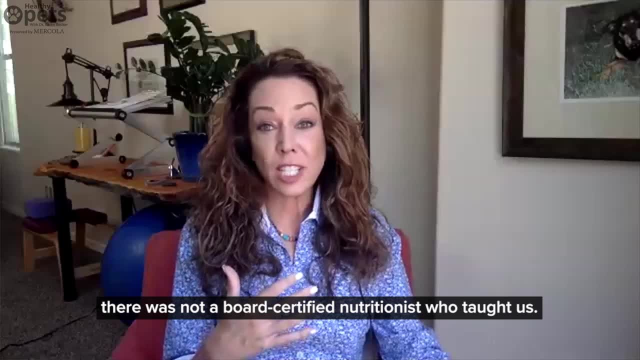 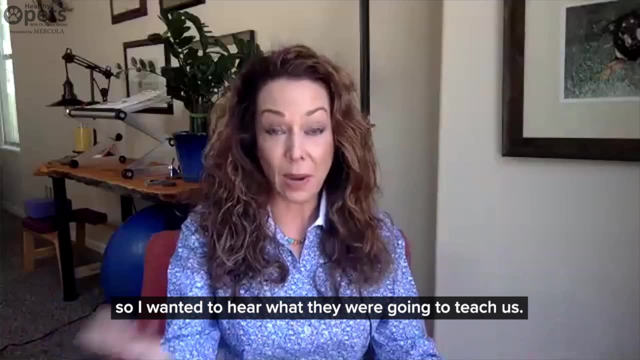 I think when I went to veterinary school there was not a board certified nutritionist that taught us. We had a rep come in and some students like totally tuned out. I, of course, I'm fascinated by nutrition, So I wanted to hear what they were going to teach us. 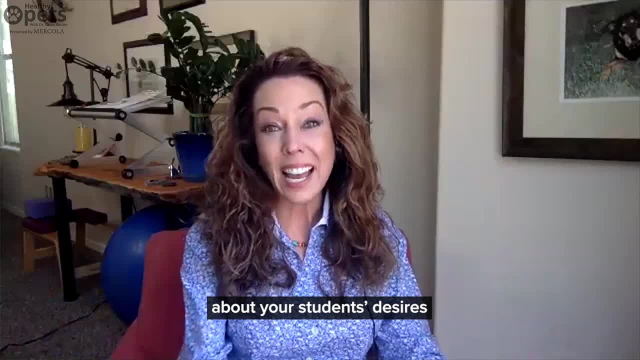 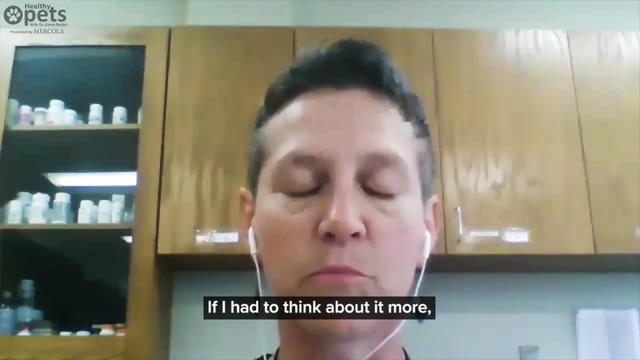 What's the barometer in the classroom about your students' desires for objective nutrition training? They are very interested, And if I had to think about it more, it's because they're relating it to themselves. There's a huge food kick on. what are we eating? 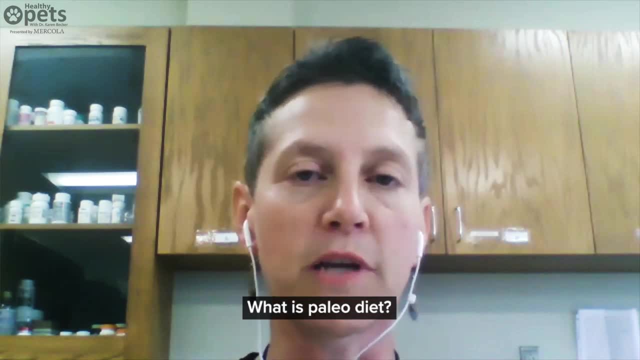 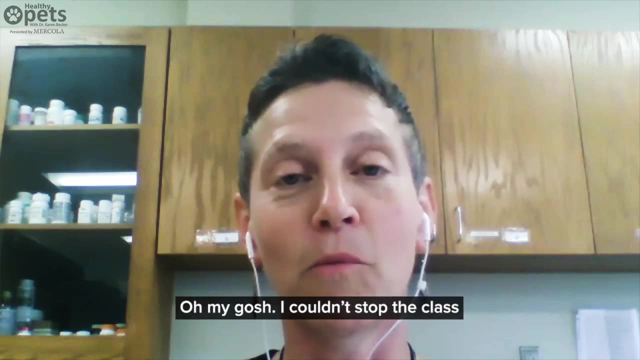 What is this? You know what is keto diets, What is paleo diets, What is fat-free diets, And so This last semester, I had a student that was a bodybuilder And, oh my gosh, I couldn't stop the class because we were talking about nutrition and 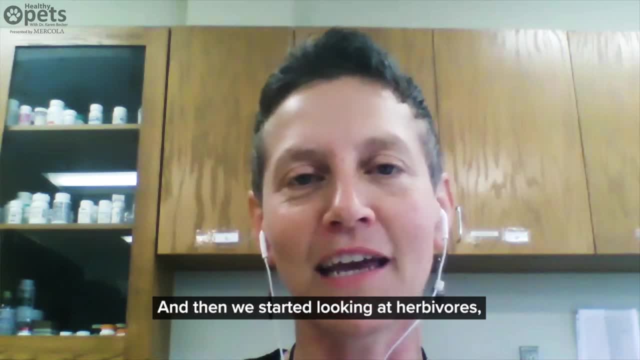 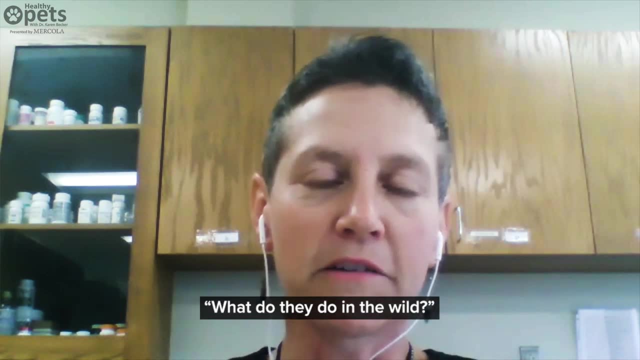 proteins and how many proteins there are. And then we started looking at herbivores and carnivores and avian And there's so many things to think about for nutrition. is what do they do in the wild, You know, even with avian nutrition, I mean, we talk a lot about exotics, is you know? 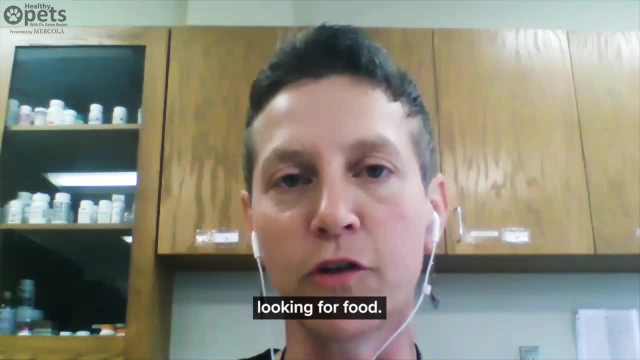 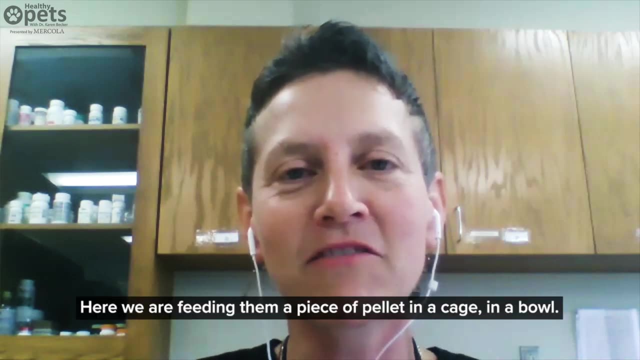 they do, what's maybe 60% of their day- is looking for food. We don't even know what they eat in the wild, whatever's in bloom, whatever's on the mountain, you know. So it's here we are feeding them, a piece of pellet in a cage, in a bowl. 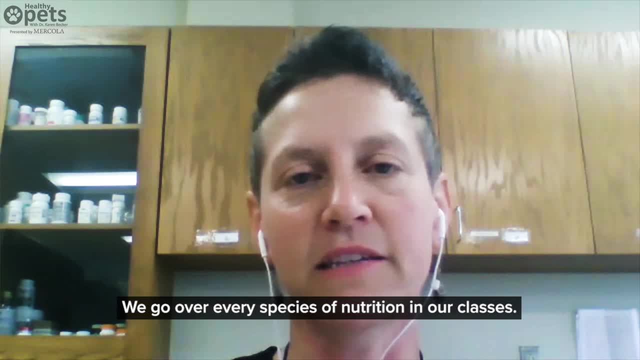 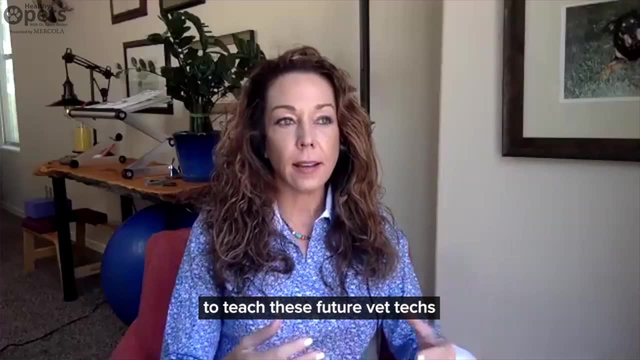 And that's not what they would do in the wild. So we go over every species of nutrition in our classes And do you? is your goal, Heather, to teach these future vet techs how to engage with clients in the exam room? 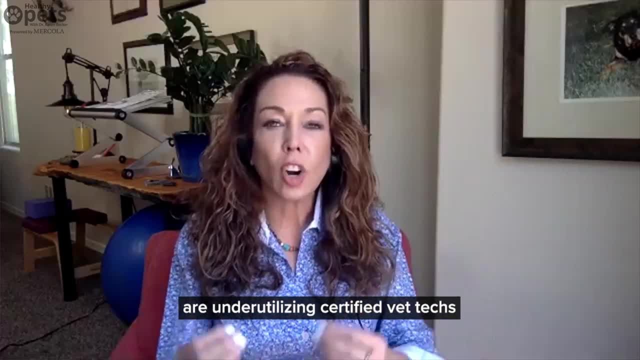 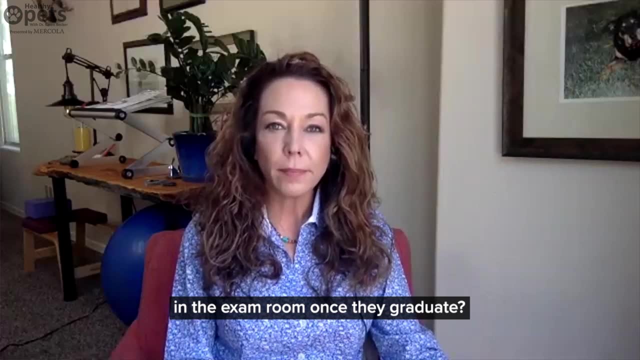 Or I guess a better question would be: do you think that veterinarians are underutilizing certified vet techs? when it comes to nutrition conversations in the exam room, They graduate. I wouldn't say more that they're underutilizing them. It's just that maybe the knowledge is not there. 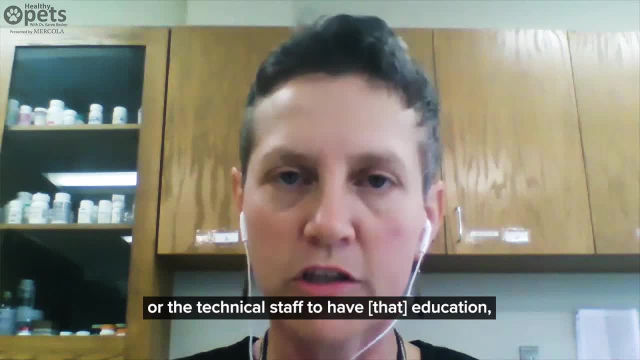 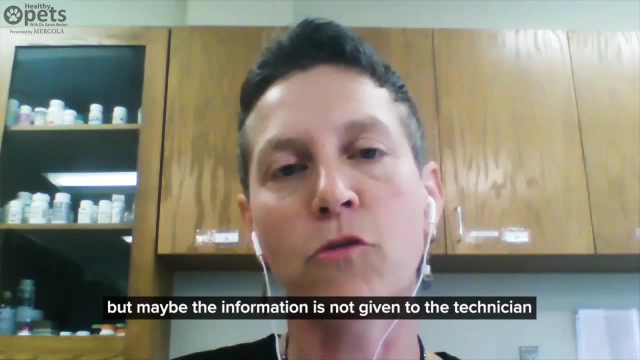 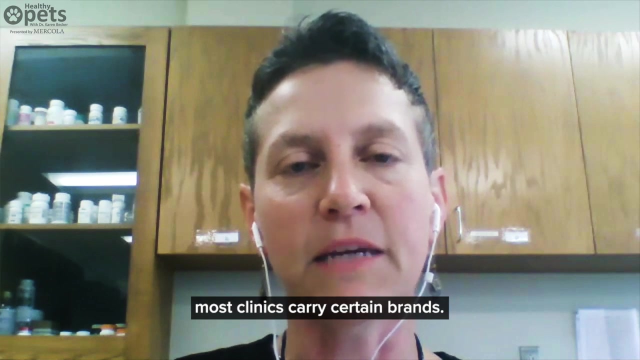 So they rely on the veterinary nurses or the technical staff to have those education. you know those talks but maybe the information is not given to the technician to provide them with a variety of options. Yeah, So in the practice you'll only see most clinic is carry certain brands. 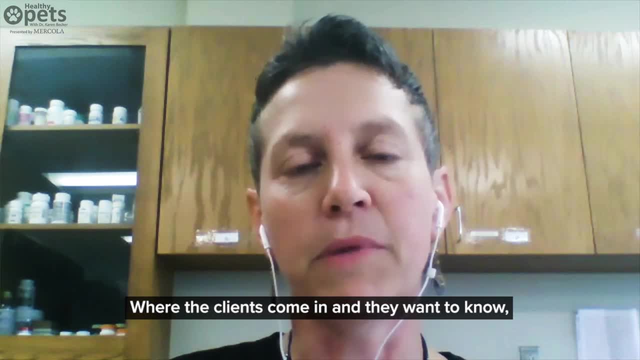 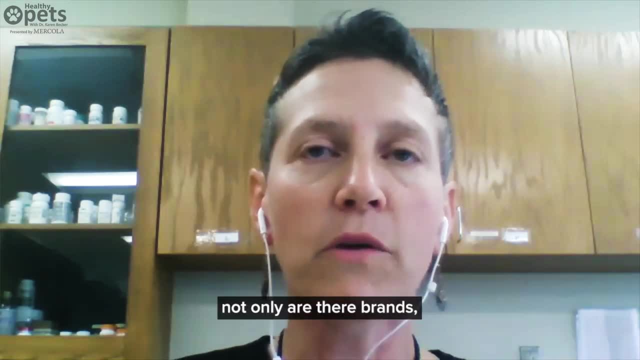 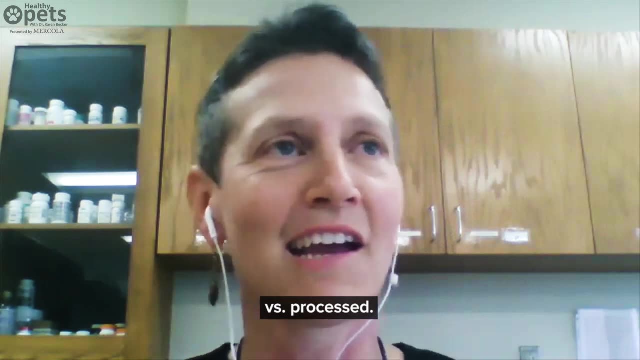 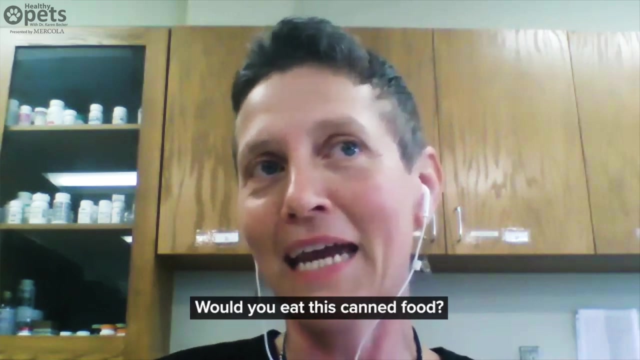 and that brand. So the students now are learning that not only is there brands, but there's also different ways, like dehydrated versus raw, versus canned versus processed. And then we go back to: what do you eat? Do you eat, you know? would you eat this canned food? 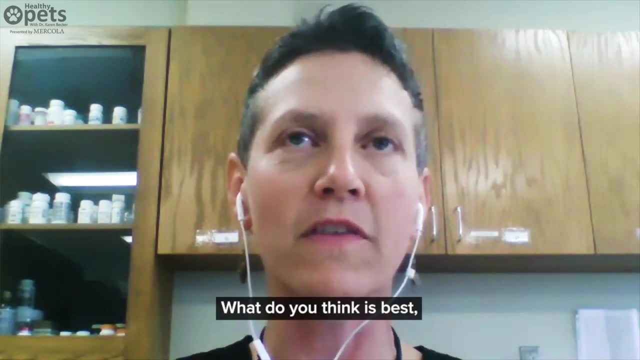 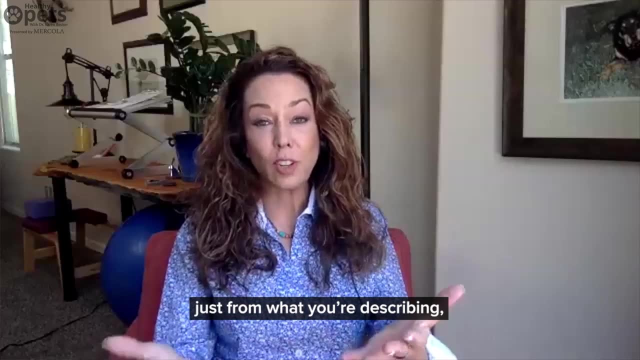 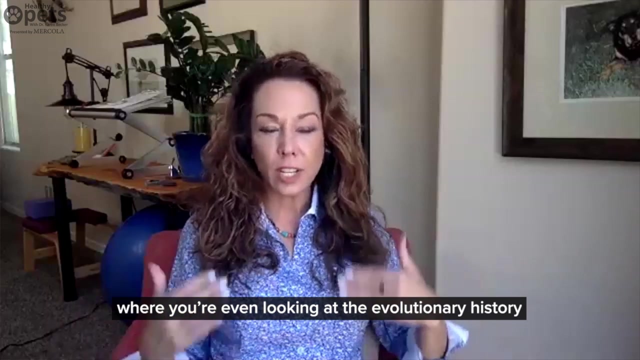 Would you eat this processed food? What would you want to eat And what do you think is best biologically appropriate for that species of animal? Yeah Well, and I think that actually, just from what you're describing, I think that your program could be one step ahead of many programs out there where you're even looking at the evolutionary history behind our domesticated pets. So I think that that's fantastic. 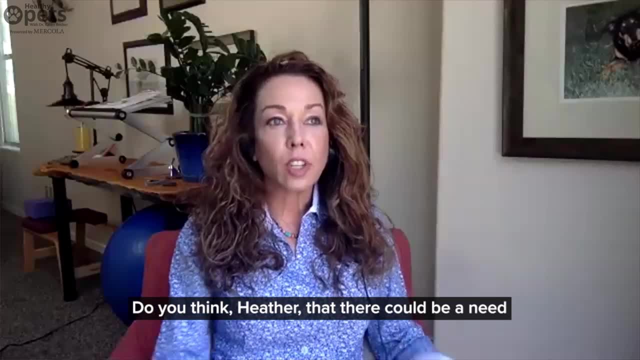 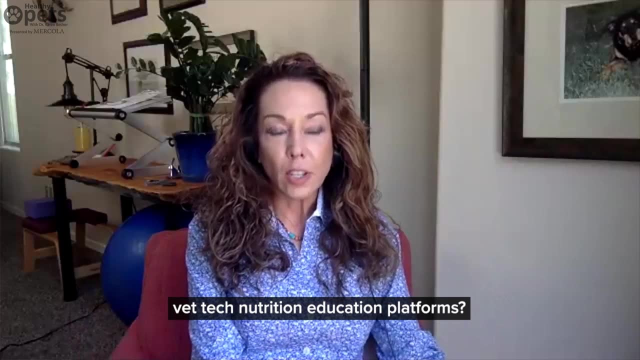 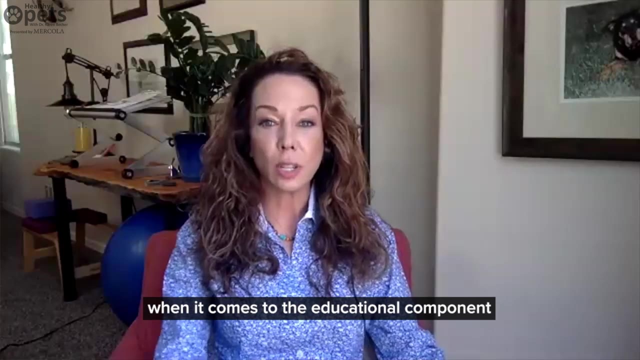 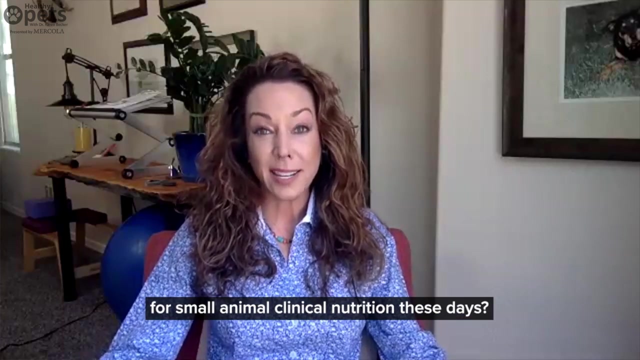 Do you think, Heather, that there could be a need or that there is a need for independent vet tech nutrition education platforms? Is there a need for additional education out there, Or how do you think that vet tech programs are doing when it comes to the educational components surrounding all of the different feeding styles pertaining to what's available for small animal clinical nutrition these days? 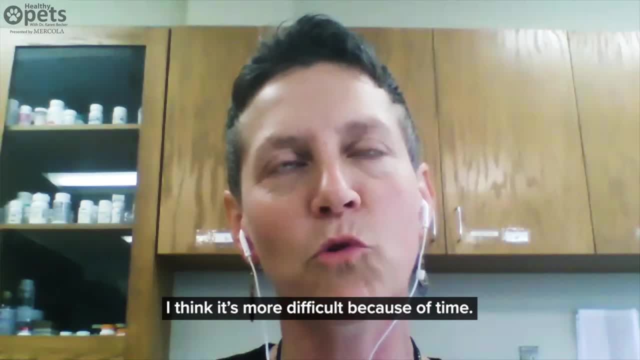 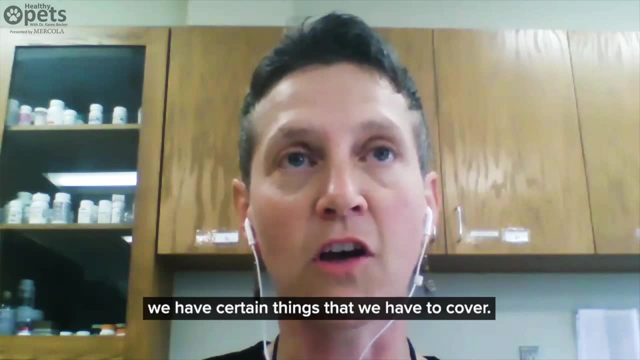 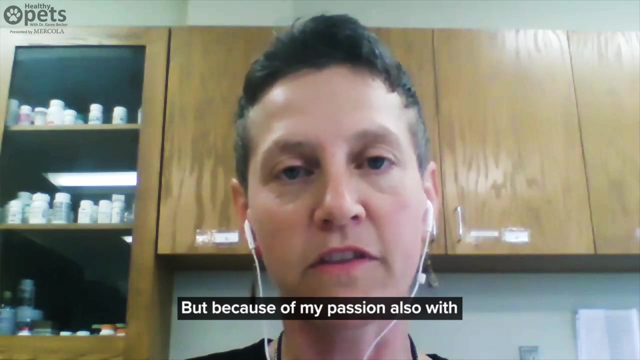 Yeah, that's a difficult question. I think it's more difficult because time- That's really what it comes down to- is. in our programs we have certain things that we have to cover. So my nutrition class: our talk is literally one day. But because of my passion also with human nutrition and animal nutrition, we incorporate it in every class. 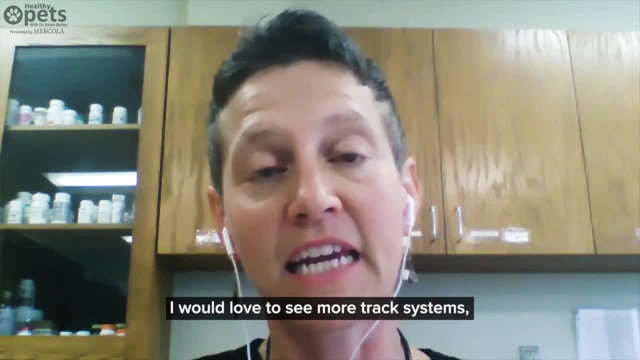 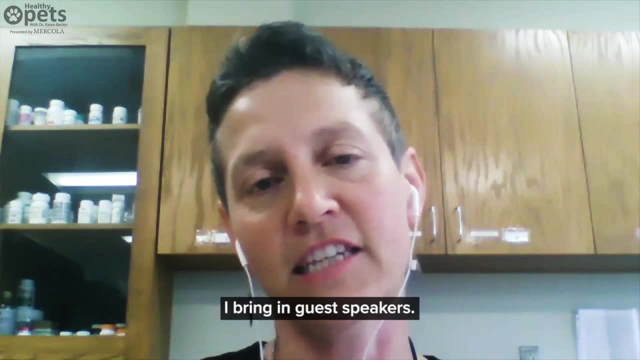 So it's more of a time aspect. I would love to see more track systems. you know where you do have tracks And in the summertime I bring in guest speakers. You know I'll have a variety of what's the topic you want to learn. 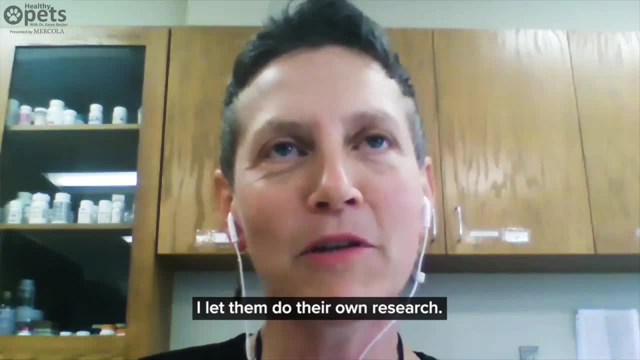 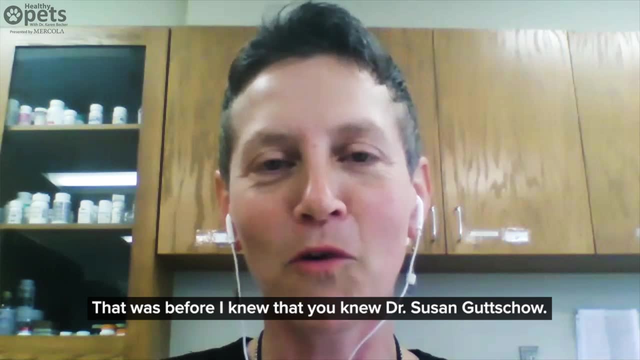 Yeah, Let's learn more about it And I let them do their own research. A funny story is that when I first started reading about nutrition, I said: let's start Googling stuff, And that was before I knew that. you knew, Dr Gutschow, And every video that I showed the students were your videos. 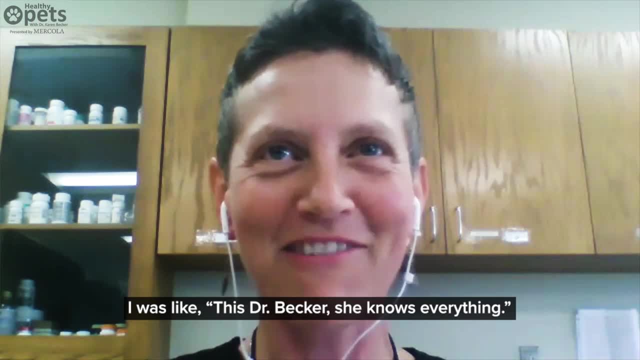 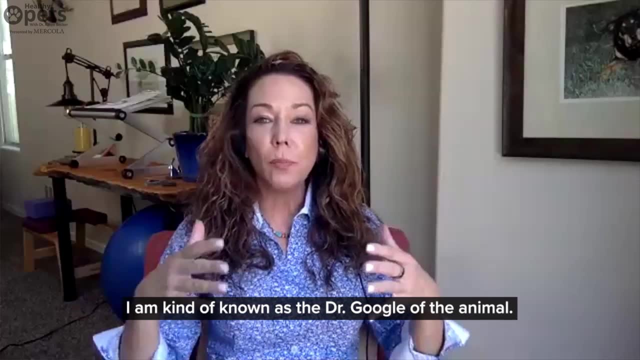 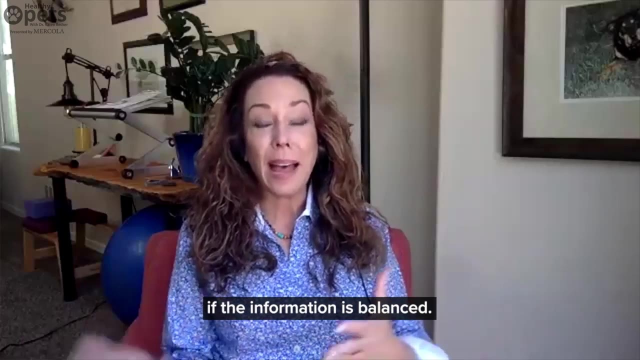 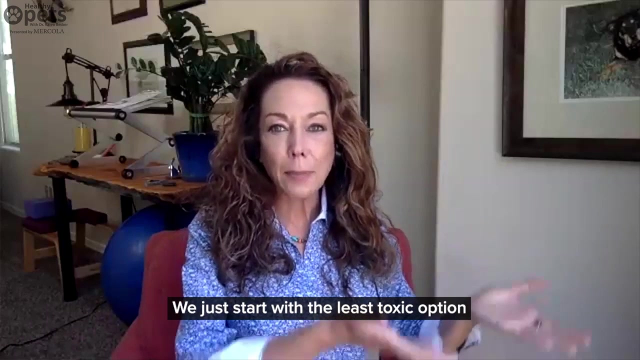 Yeah, And I was like this Dr Becker. she knows everything. Well, you know, it's interesting because I think by default I do. I am kind of known as the Dr Google of the animal, And that can be a blessing and a curse if the information is balanced. And of course, I try and be very, very balanced in providing what I what I call common sense approaches, which is, start with the least toxic option and move to toxicity.